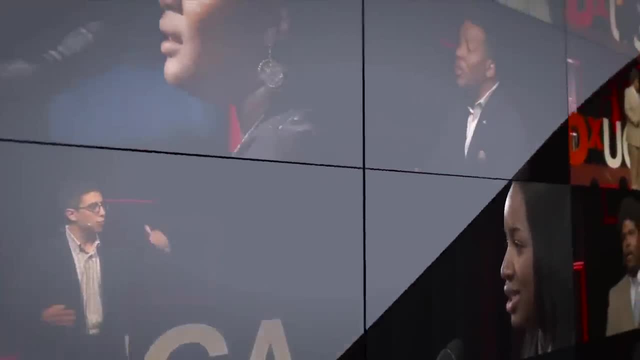 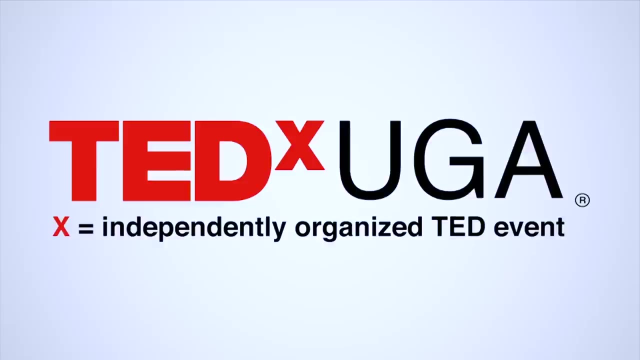 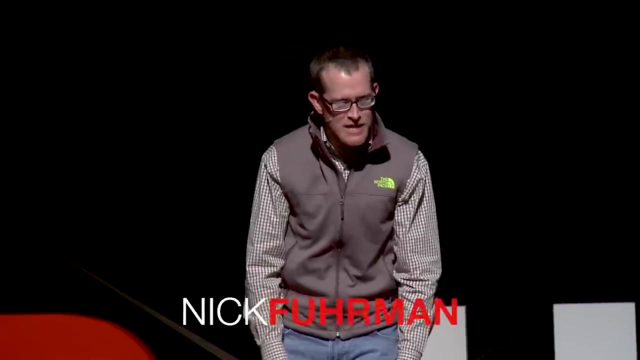 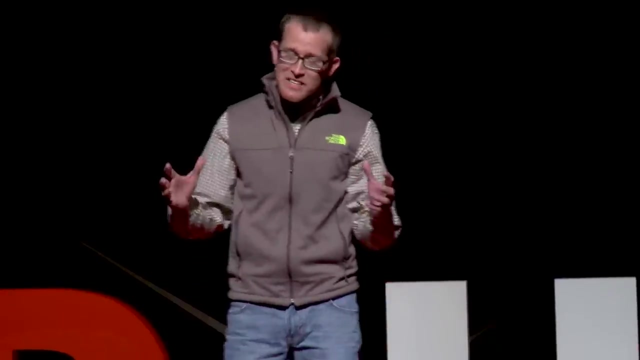 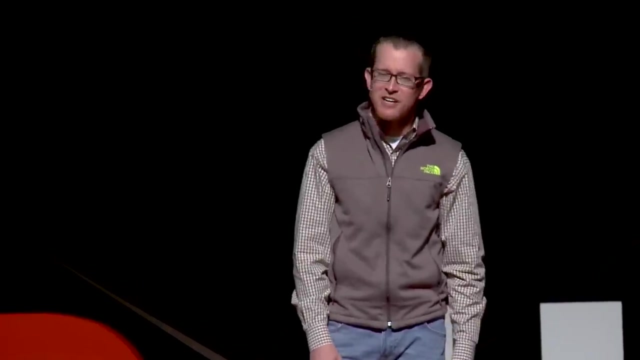 45 minutes: That's the amount of time it can take to change somebody's life forever. It happened to me. I'm going to take you back to Maryland and me as a seven-year-old. I grew up in Perry Hall, Maryland, and I'm sitting on a carpet square on this particular Tuesday. 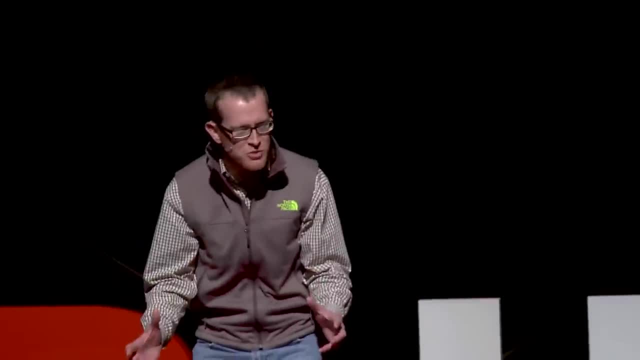 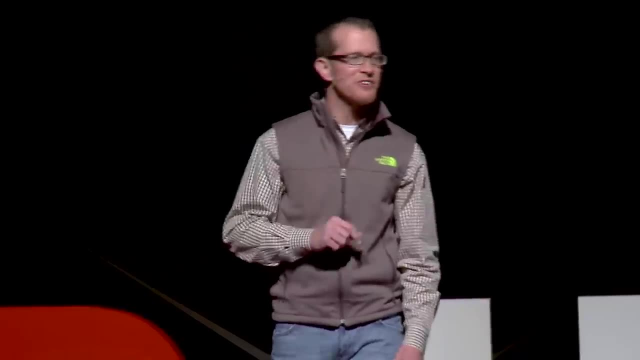 morning in elementary school and I was on the edge of the carpet square And my friends and I were all on the edge because there was a guy who was coming to visit our school on this particular day who was known as Ranger Bill. Ranger Bill worked for the Maryland. 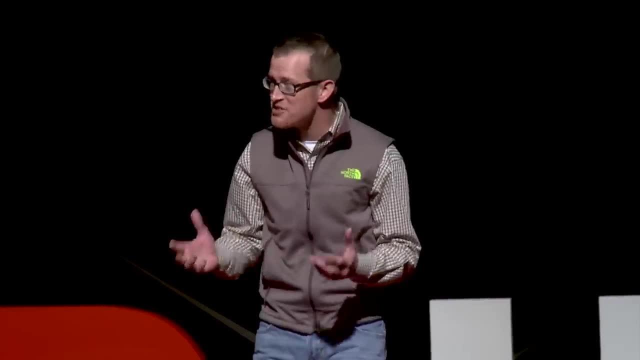 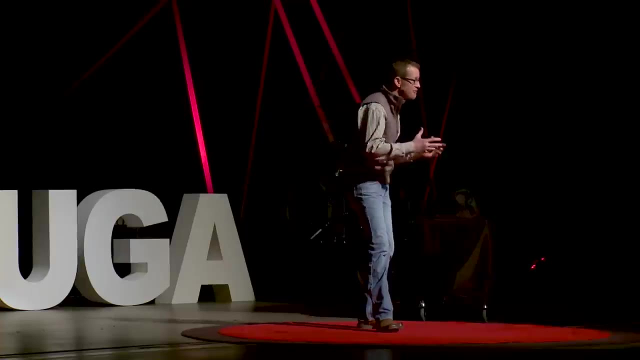 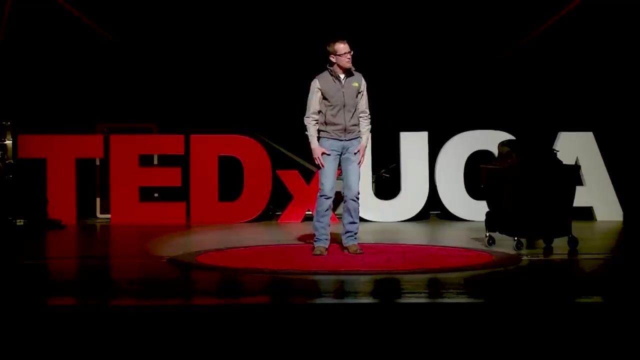 Department of Natural Resources and Ranger. Bill was an environmental educator And he brought with him that day a turtle and a snake and an owl and a hawk and a vulture And he came in and this guy was looking snazzy. He had this great-looking uniform on all these animals. 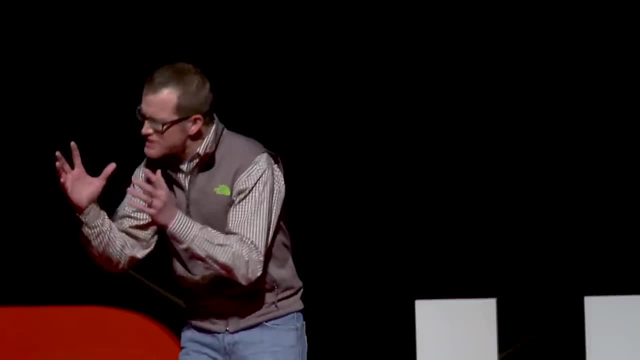 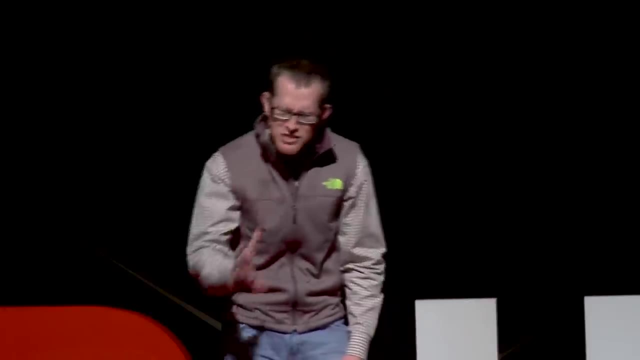 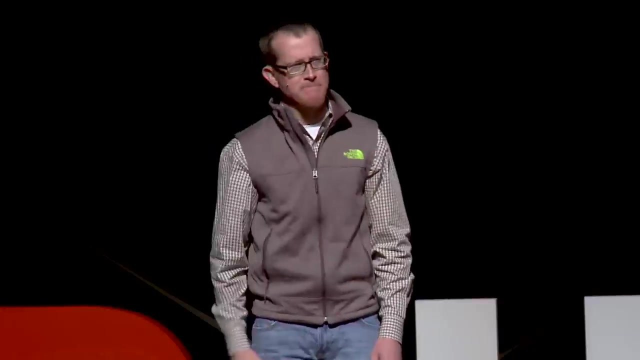 and he edutained us. It wasn't just teaching, He was entertaining us. He had us on the edge of that carpet square And I watched this guy teach this day and I remember 45 minutes is the amount he spent with us. and then he left And I remember thinking to myself: I want to be like 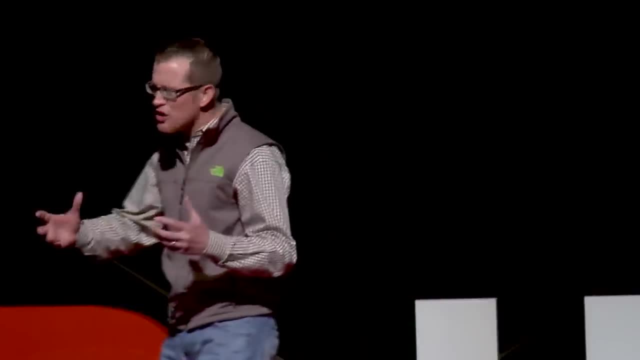 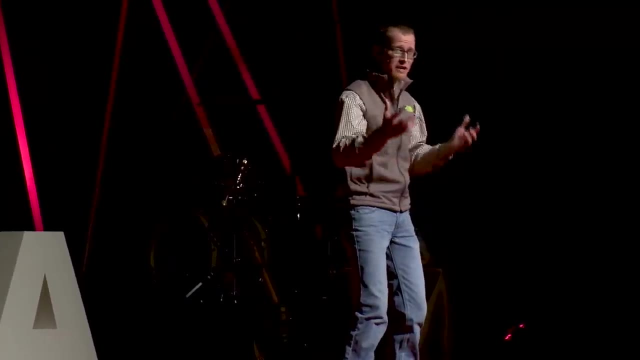 that guy. I want to be like Ranger Bill: the way he looked, the way he was teaching everything and the animals he was using. All these animals had injuries and they had stories and they were ambassadors of the messages that he was sharing. Well, I went home that day and told 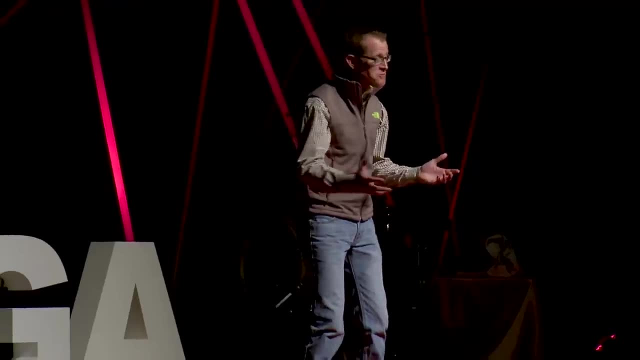 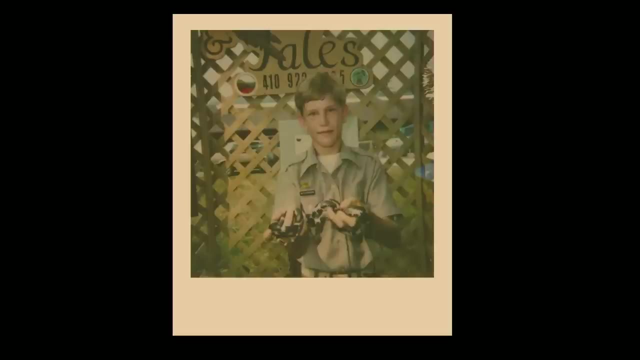 my parents about it and I guess I kind of became a Ranger Bill groupie because I went out and I started following this guy around- Probably wondered what is this little kid, this seven- or eight-year-old kid, doing in the back of? 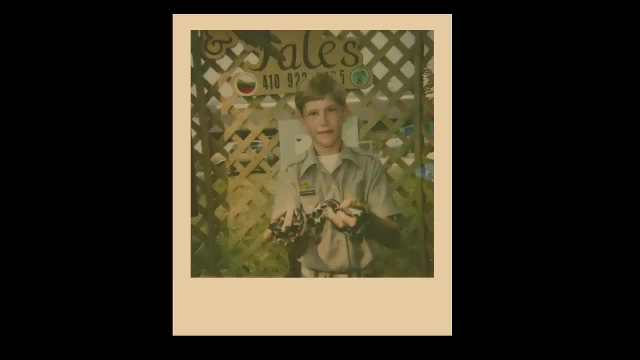 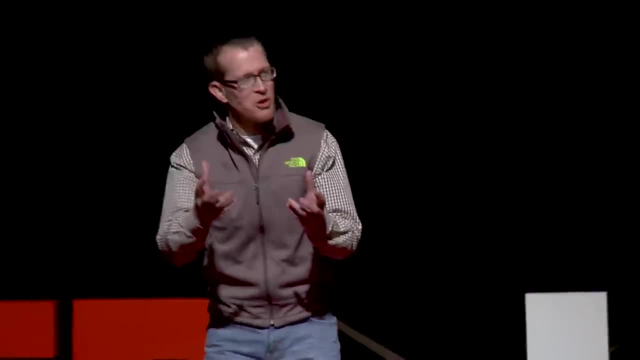 the room watching me everywhere I go. He'd go to the library. We'd go up there and see him- All these things that picture there with little Nicky there, Ranger Nick with the uniform holding the Eastern Kingsnake. You know, I finally got up the courage to go up and talk to Ranger Bill. 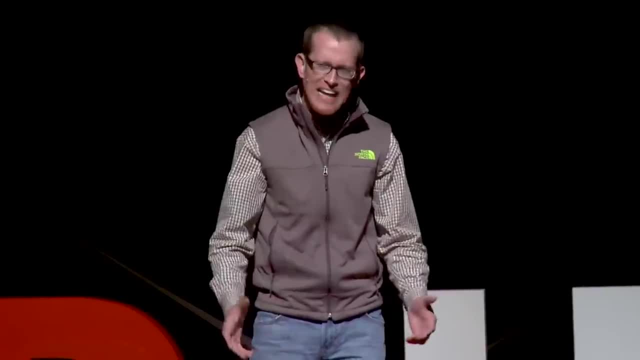 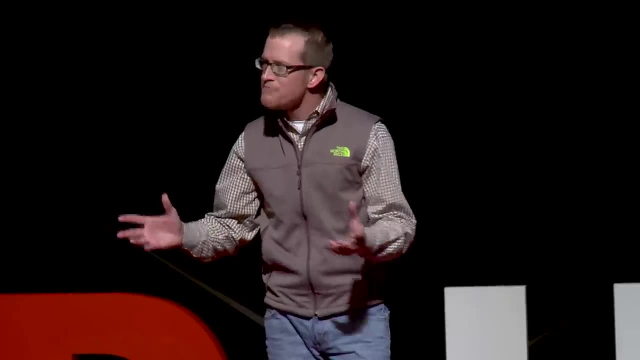 even after doing the junior Ranger program with Ranger Bill- And I'm about eight years old at the time- and I ended up saying: is there anything that I can do to help him? And I said, well, I'm going to help you, to be around you more, to shadow you, to help you. And I tell you what he said. He said: 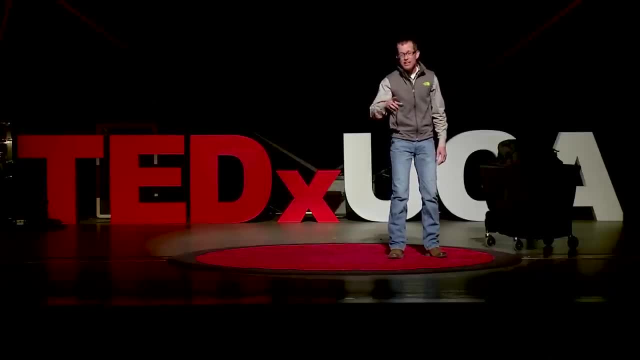 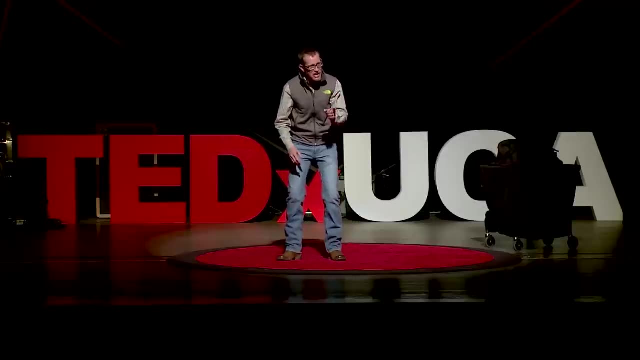 well, you sure can, And I ended up for about the next eight years cleaning a lot of cages out- all right, And owls and hawks are not the cleanest animals in the world- but I got a chance to be around this guy and watch the way he was teaching And I'd go out with him on the stages in different 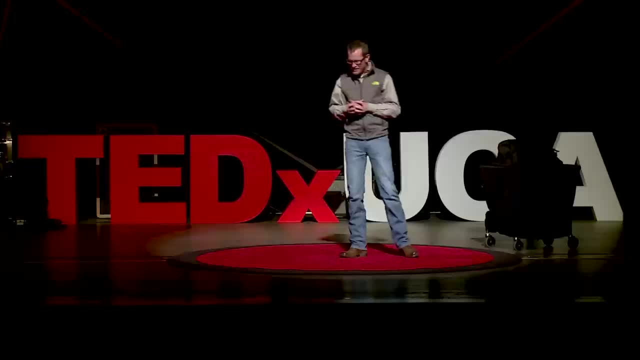 places and watch him teach. And after a little while- maybe I was 11 or 12, he'd say: Nick, why don't you hold this turtle and stand up and talk about it a little bit? Or Nick, why don't you hold 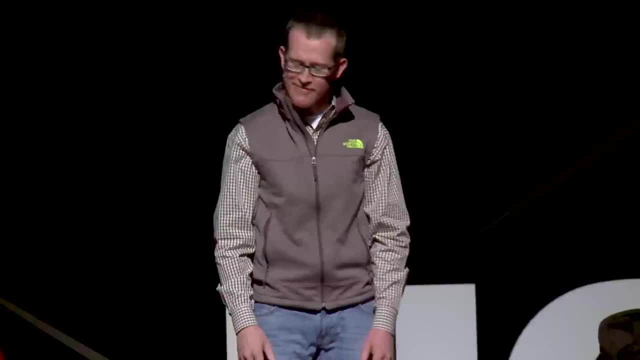 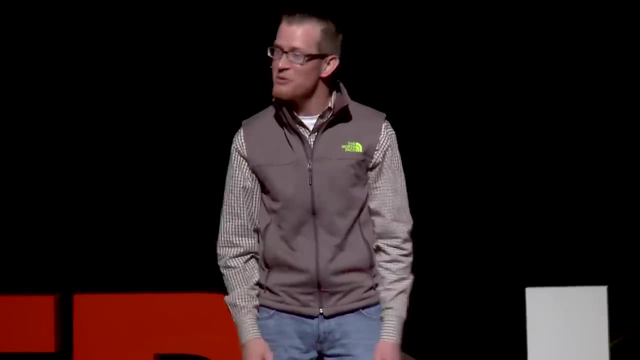 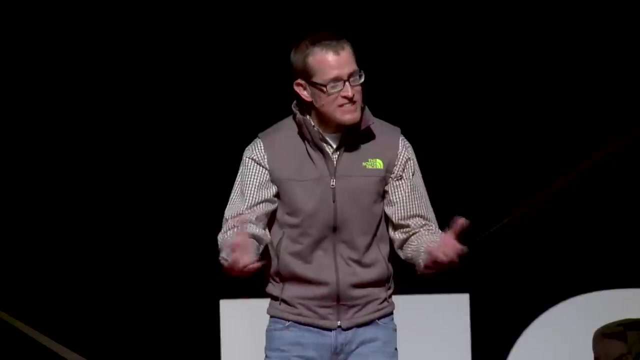 this Eastern screech owl and tell the audience about it a little bit. I did that stuff and I turned 16.. And Ranger Bill says to me I'd been doing this eight years, going out and talking. and Ranger Bill says, Nick, this is all you've ever known is watching me teach and wanting to. 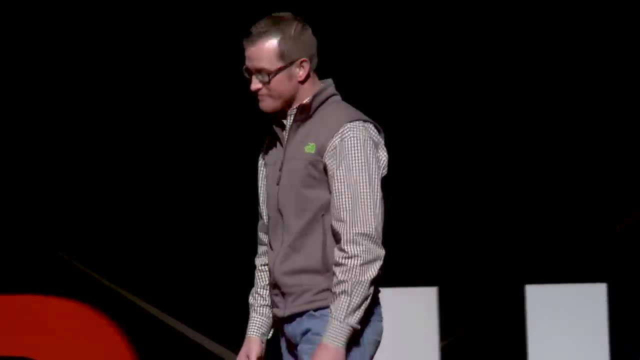 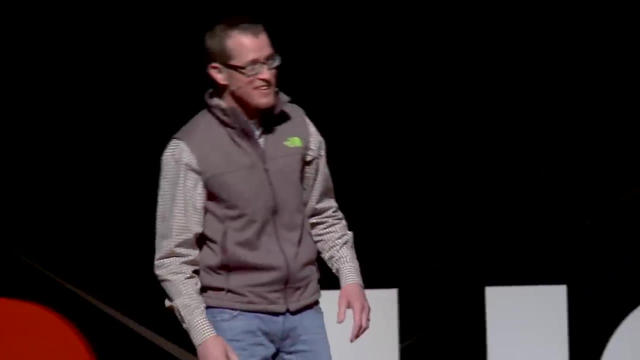 teach with animals. He said: why don't we offer you a job? So I was the youngest guy working for the state of Maryland, the Department of Natural Resources, this little 16-year-old kid with my Ranger uniform and everything, And I would start going out there and using animals to teach with. 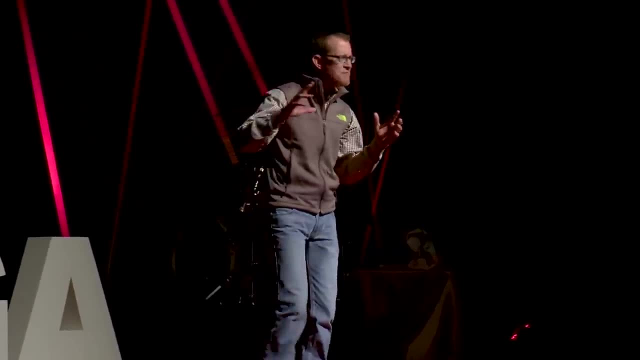 Now you had to be 18 to drive a state vehicle, so I had to drive my old Chevy Blazer. I'd put the seats down in the back, I'd put those carriers, the birds, in there and we'd go out and I'd talk. 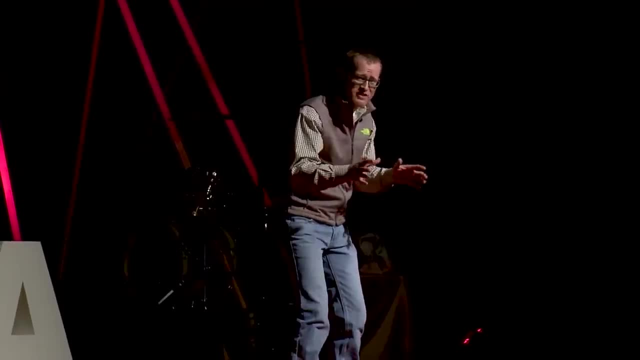 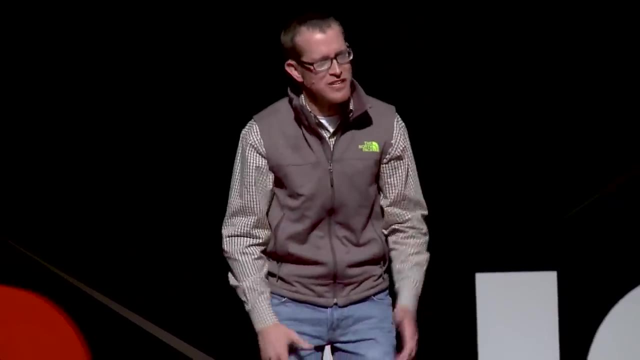 Now I couldn't teach a bunch of high school kids. I was younger than they were. You weren't going to listen to me, But I could go out and I could teach younger kids And I'd visit camps and things and use animals in teaching. And I remember one day- it was in November- 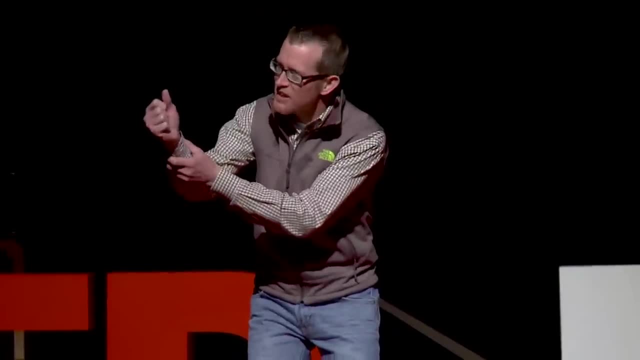 sometime I was at an event and I was holding an owl on my glove over here And I remember a news guy came up to me And he had a camera there and he put it in my face and he said: I'm standing here. 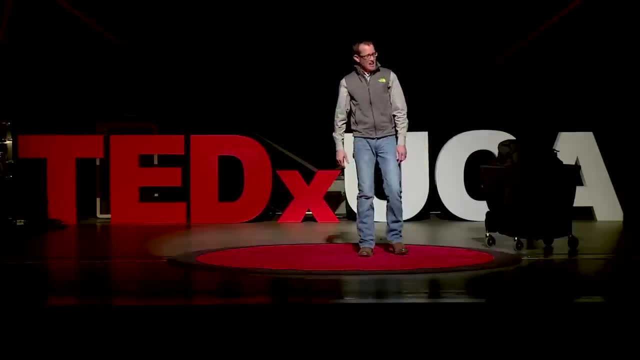 with Ranger Nick And when he said that I felt like I had really made it. you know, Like I had man. I yeah, My whole life. this is all I'd ever my great-grandmother used to say you really. 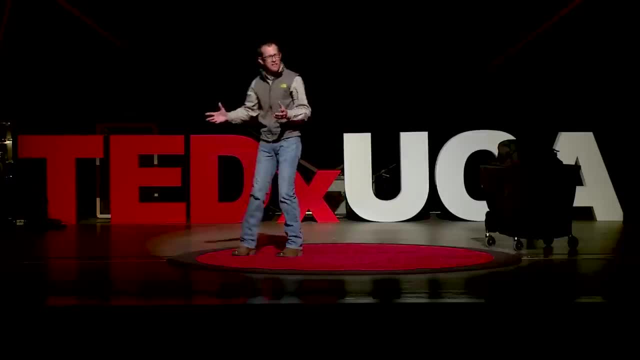 called me your little preacher boy. And if I didn't think I was going to be a preacher boy, I didn't do this Ranger thing. I'd probably become a preacher. And people say, well, maybe you ought to think about doing that, But I didn't. And I that guy called me that And it was a profound. 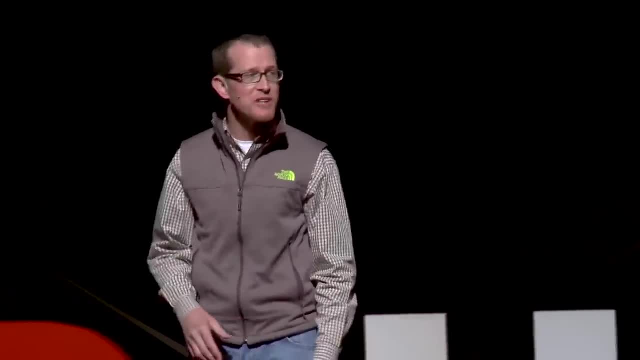 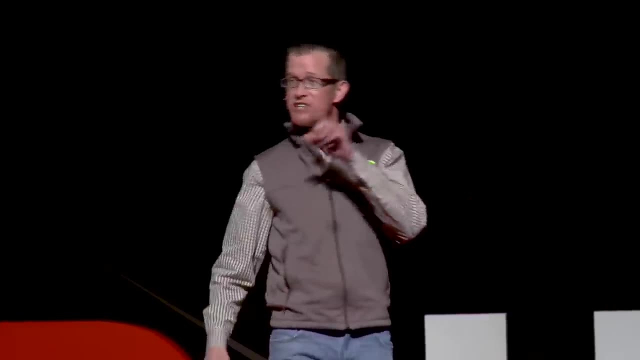 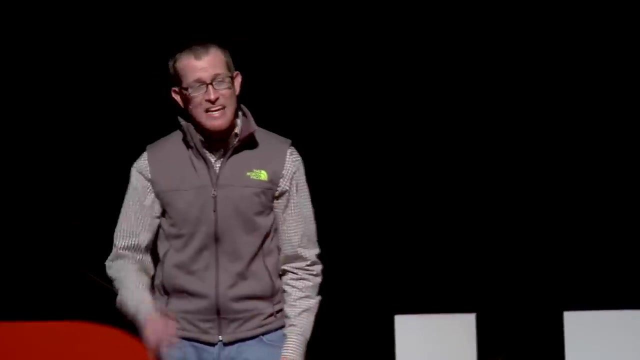 moment. Well, I continued teaching with those animals for a number of years, And that led me down a path to college and graduate school and at the University of Georgia now for 10 years, teaching students how to do what Ranger Bill did 31 years ago- Still talking about it, And he was. 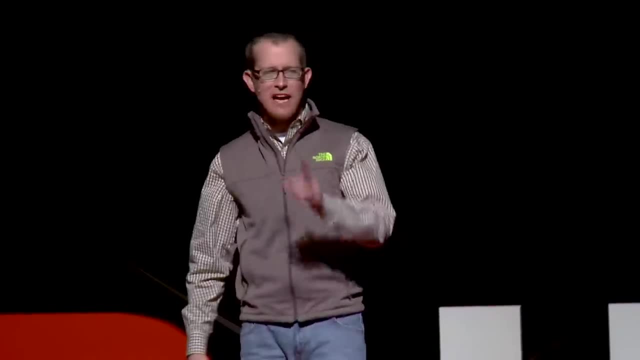 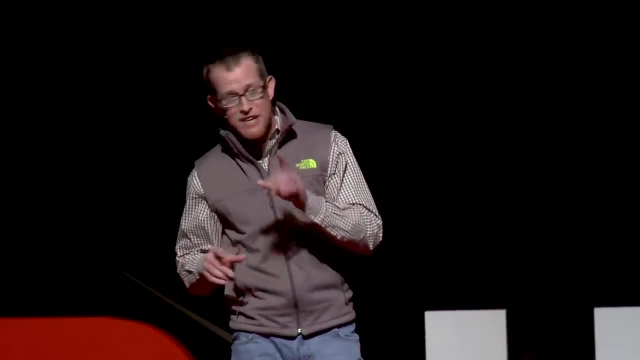 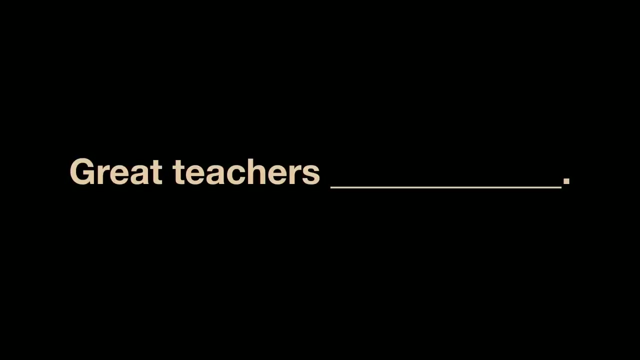 there for 45 minutes- Profound impact. Ranger Bill wasn't just presenting information, He was teaching it. And there's a difference. I want you to think for a second about a great teacher in your life. What would you put in that blank? Great? 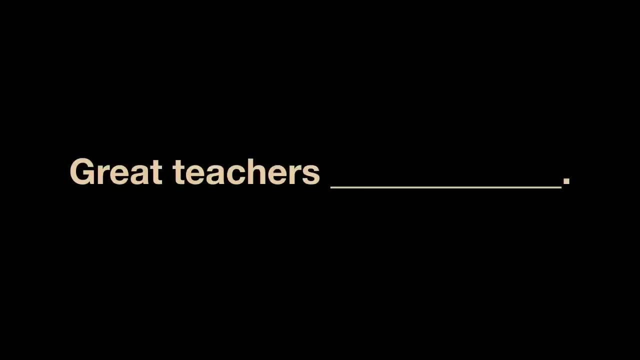 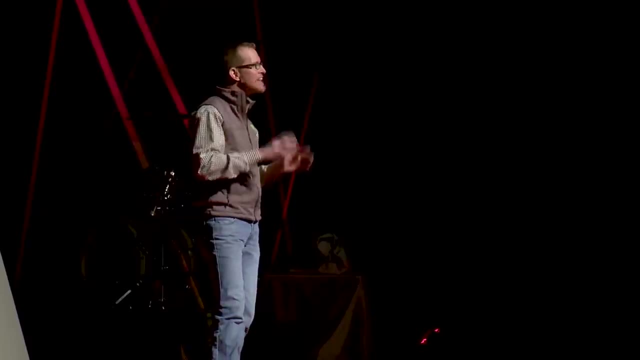 teachers what Think about it? I'll give you seven and a half seconds. No cheating, Keep it to yourself. I'm going to come back to it in a couple minutes. I'm going to talk about that Because I have my own thoughts about what great teachers do. 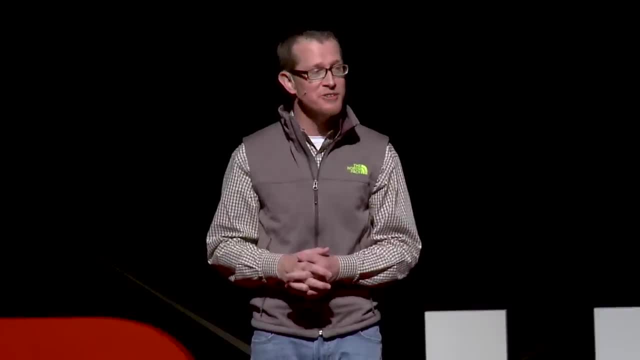 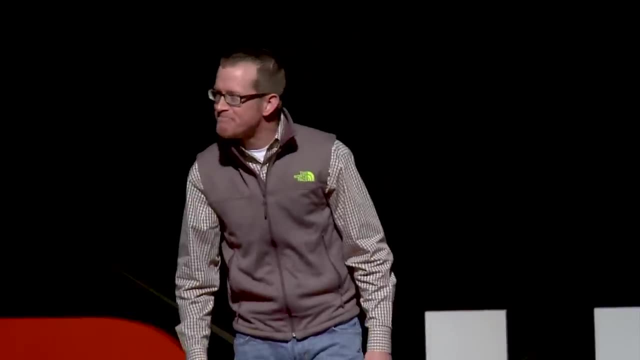 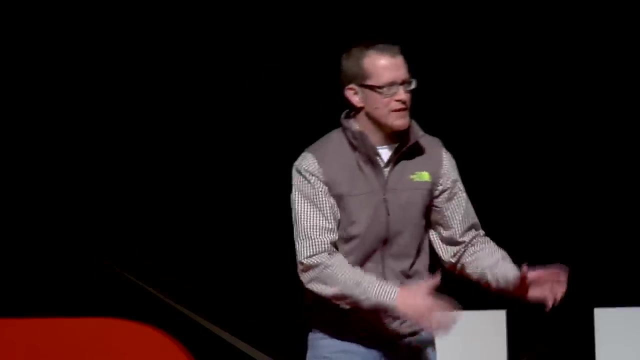 The first thing that I think great teachers do is they celebrate mistakes, Errors, Things that happen that weren't planned, that we have a choice as an educator whether to capitalize on this or ignore it. Bob Ross, that television artist that paints things on TV, calls them happy accidents. 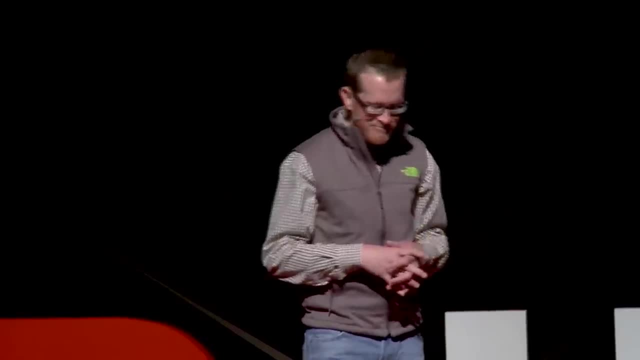 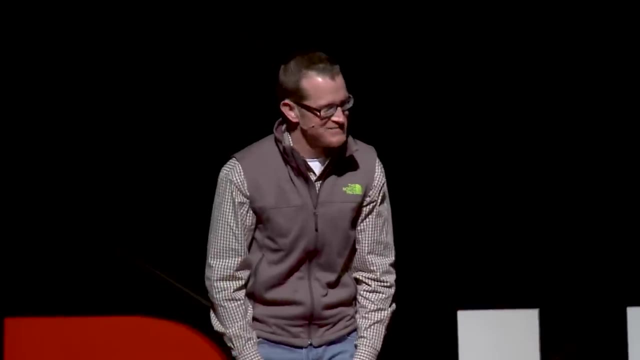 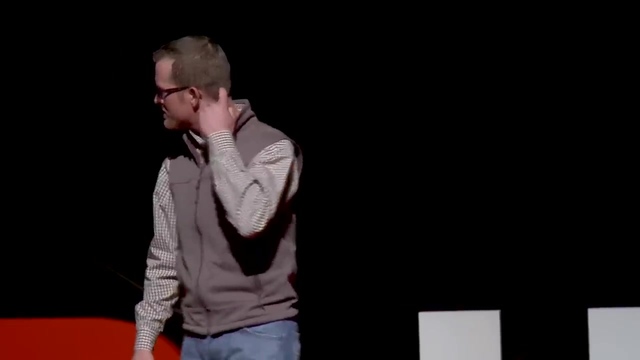 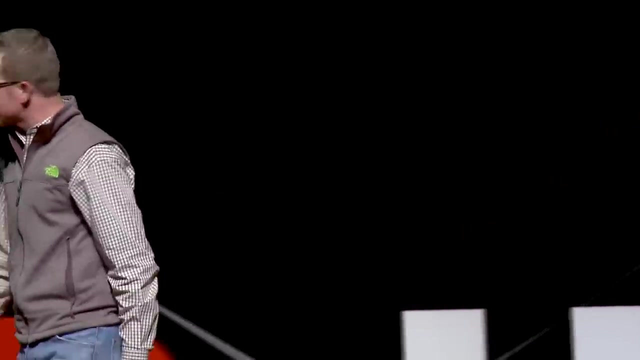 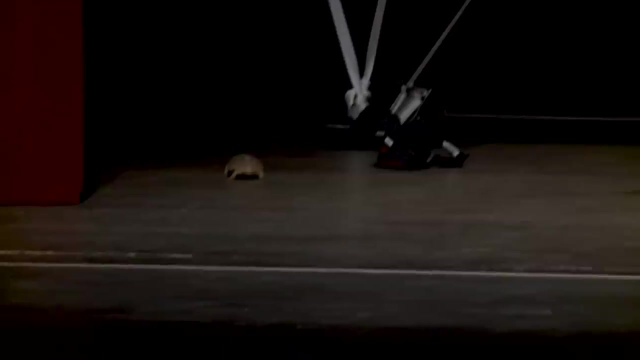 It's a happy accident we made here. Okay, In the education world we call these things teachable moments. Just makes it sound better. You make a mistake. you call it a teachable moment And sometimes, from time to time- I don't know if y'all, I don't know if y'all see this or not- I know I'm not supposed to leave the rug, but something's going on over here. I hope they forgive me. I'm going to come over here Talk about a teachable moment. Look what's going on right here. This You're not going to hang. 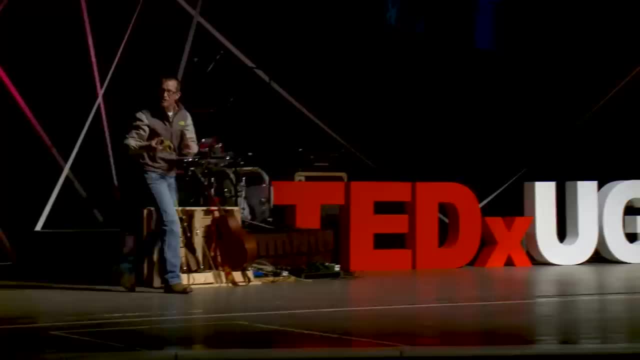 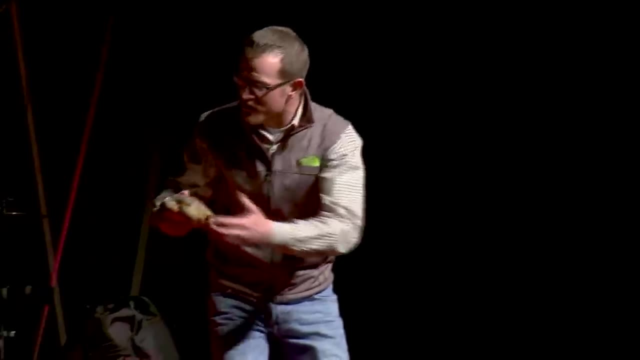 What are you doing? What? You're not going to believe this. Not that this was planned or anything, But all of a sudden I look over there and there's our state reptile, A gopher tortoise. We're talking about teachable moments. 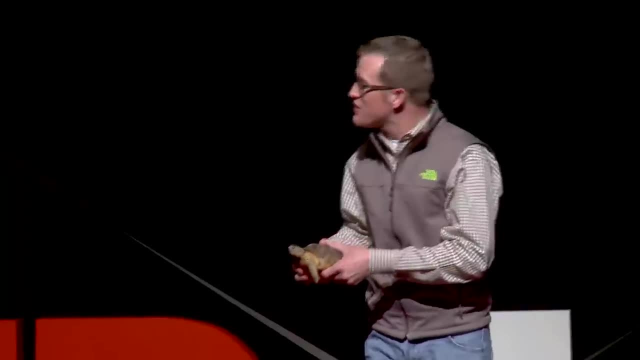 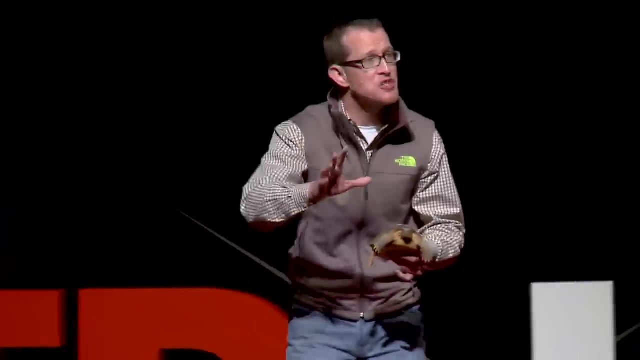 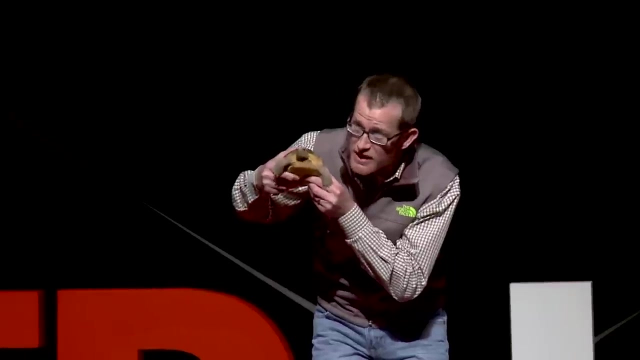 I had a choice to make right now. I could have either ignored that and continued on, or it could have become a distraction, And so I thought let's capitalize on it. It's a teachable moment. if you don't mind indulge me for a second, Let me tell you a little bit about Shelly, Okay. 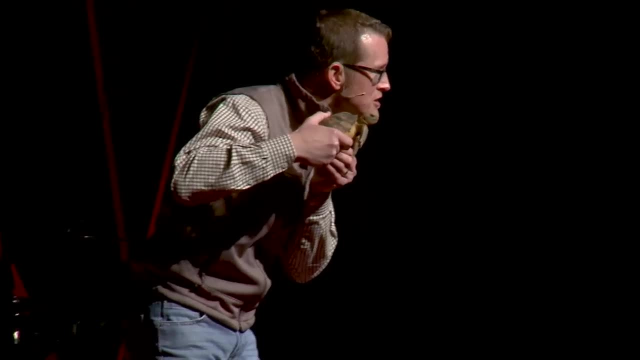 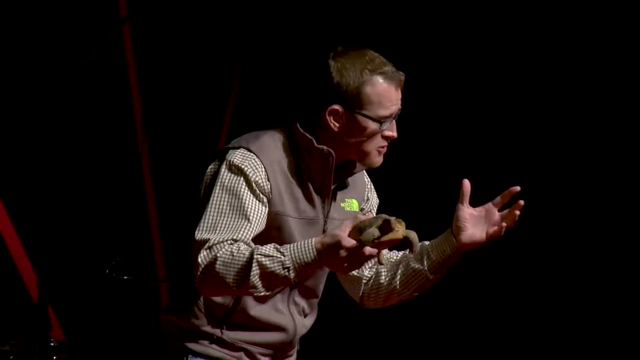 this is Shelly, And look at the face. I mean, is that not the cutest? Shelly is 12 years old. She'll get almost 100 years old. when she's at her maximum lifespan, She'll get about three times. 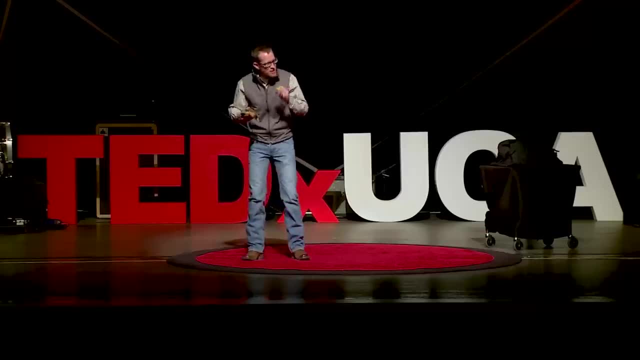 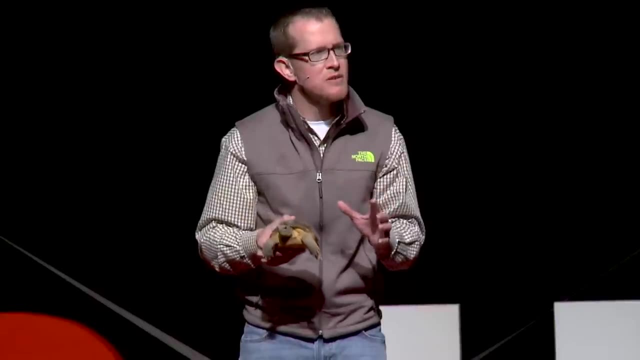 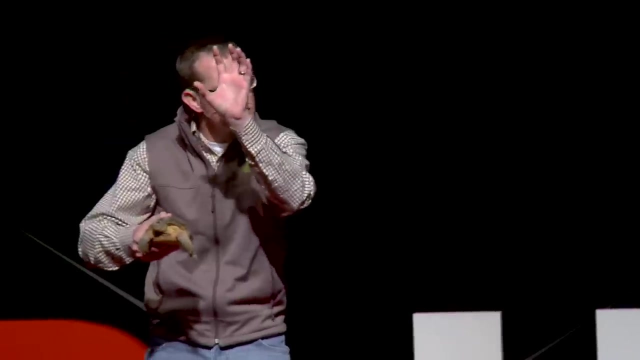 this size. Shelly is a gopher tortoise, a state reptile. A lot of people didn't know Georgia had a state reptile. That's pretty cool. She is a keystone species Man. that sounds important And it is Just like an archway: has a bunch of stones on it and there's one stone at the top that holds. 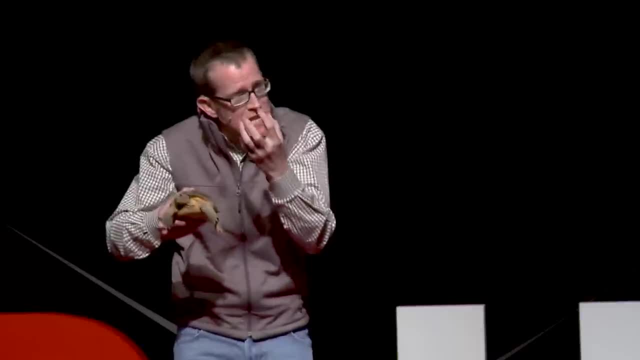 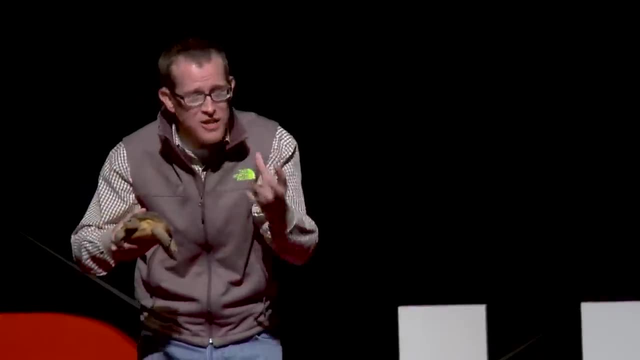 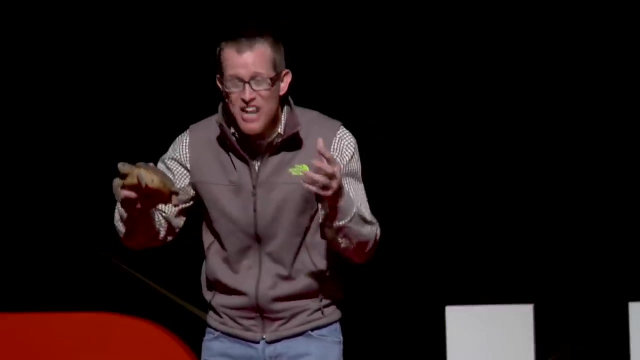 all those other stones in place. If you take that keystone at the top away, all the other stones fall down. You take this little lady out of an ecosystem keystone species. all these other animals are going to be impacted Because she digs these gigantic burrows in the ground that are the size of a school bus. 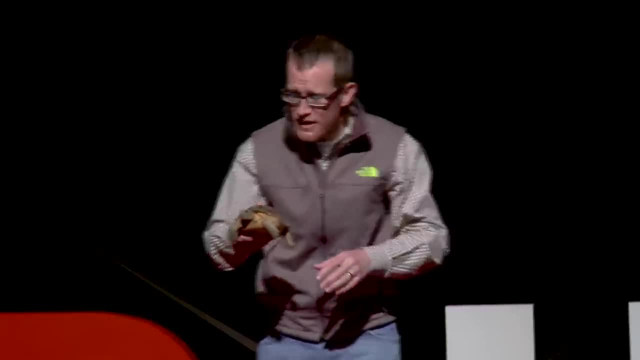 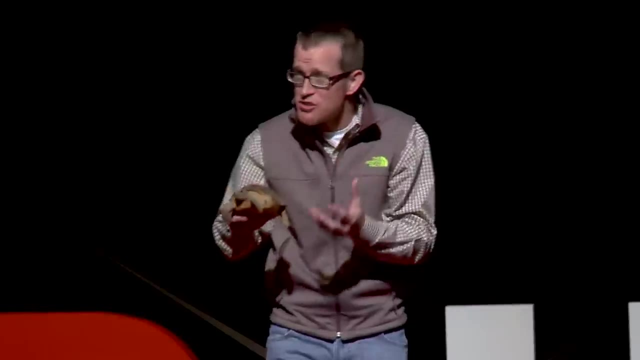 And when fires come through in South Georgia and North Florida, all the animals that the fire would otherwise burn up, these animals go into her burrow. So she is essential in an ecosystem and she is a species of concern. right now These guys and gals aren't a whole lot out there anymore. 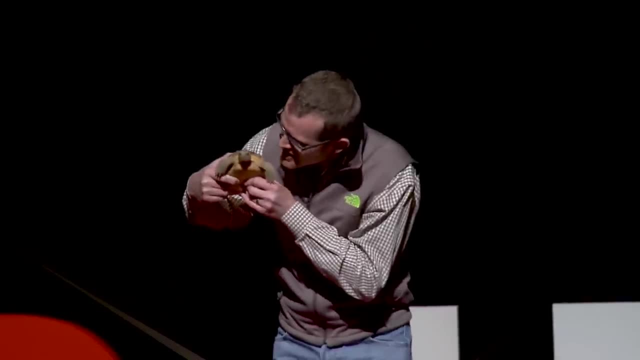 so we got to do what we can to help them. So I'm so glad that she decided to make a little entrance. Every once in a while she'll kind of wave: Oh look, she's waving at you, Look, look. 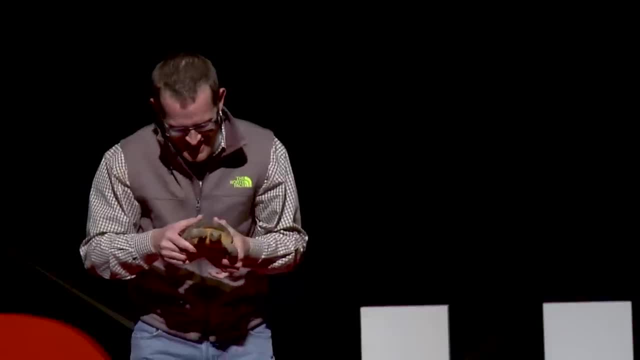 You do that to kids and the kids, everybody's waving back. you know, That's just something else. All right, lady. Well, I tell you what I'm going to get. this Becca is going to come out here. 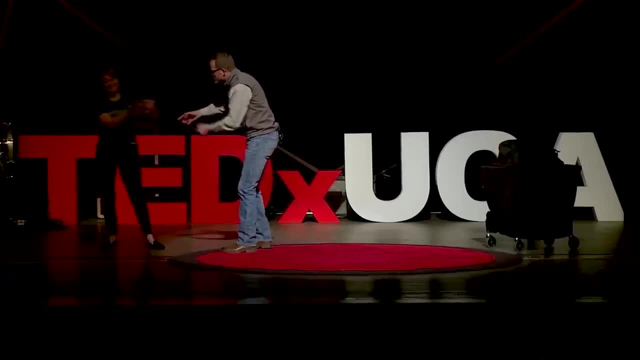 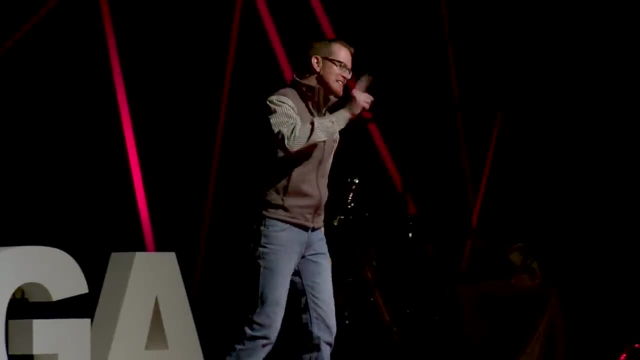 a turtle herder. Thank you, Becca. I'm going to give her back to you. Look at that, She's frisky. now Be careful. Yeah, Celebrate mistakes. Next time you make a mistake, call it a teachable. 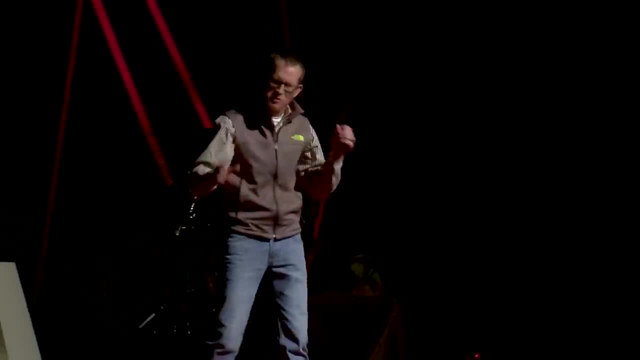 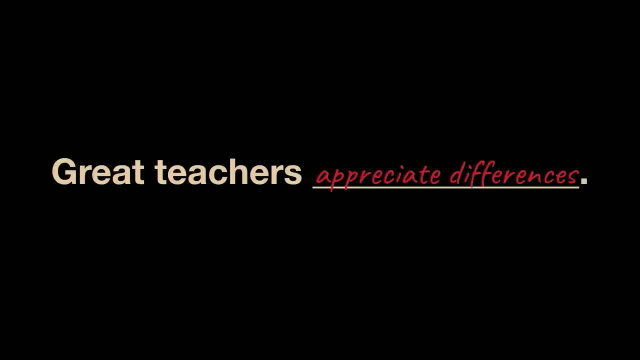 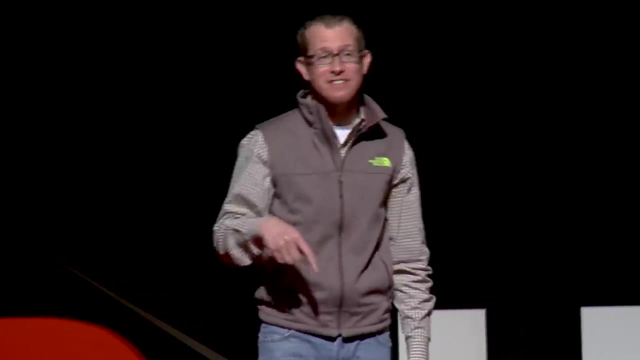 moment You'll feel a whole lot better about yourself. That's a teachable moment. First thing great teachers do is they celebrate mistakes. Second thing I think they do is they appreciate differences, And I don't need to tell you that, as a professor at UGA, I got a lot of different kinds of students in my classes. 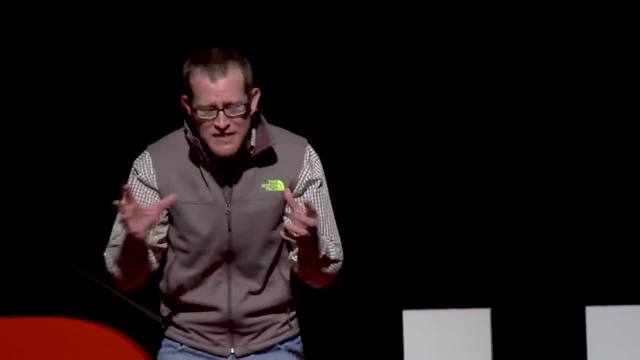 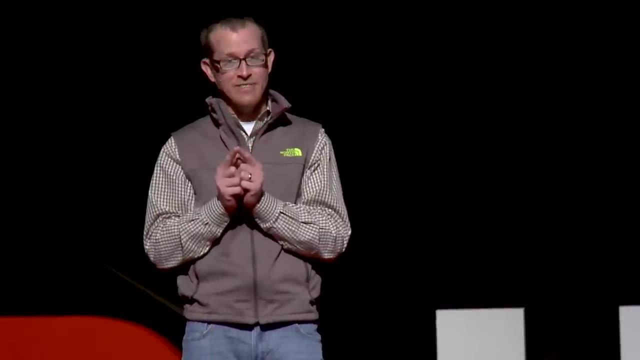 Everybody's different, And that's great because they bring all these different perspectives and levels of experience into that classroom, But every one of them has something in common, And every one of them has something in common, just like most of us do in this room tonight. 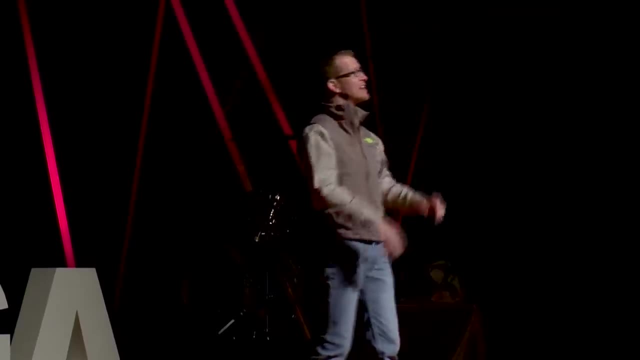 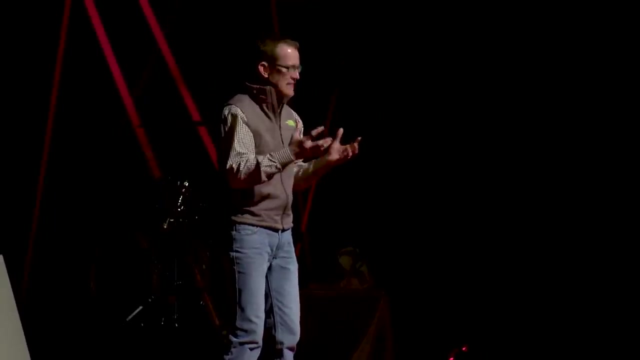 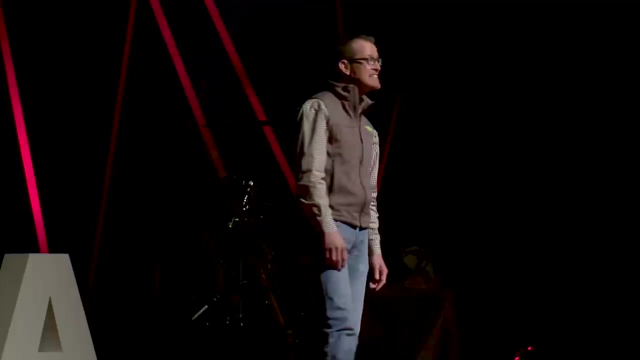 Everybody deals with public speaking anxiety, Sure Communication, anxiety, And the students that are in this class come into this class with me that I call teaching with animals, And it is just what you can imagine: A class about teaching with animals. We learn about public speaking, but we 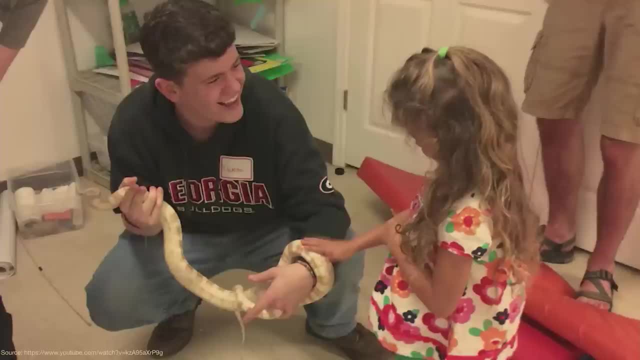 integrate animals, like that animal in that picture, and help students overcome anxiety by handling an animal and teaching with it And they'll tell me: I'm going to teach with an animal, I'm going to teach with an animal And they'll tell me. they'll say: Ranger Nick, they'll say when I'm holding: 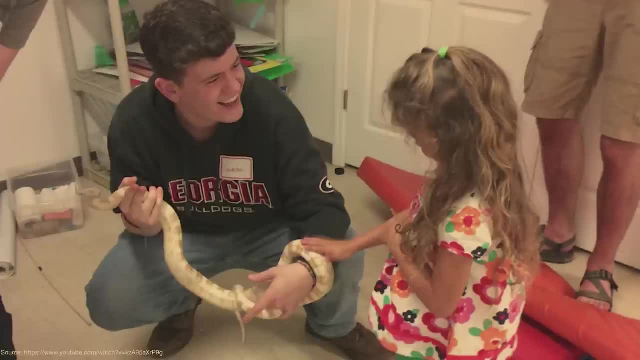 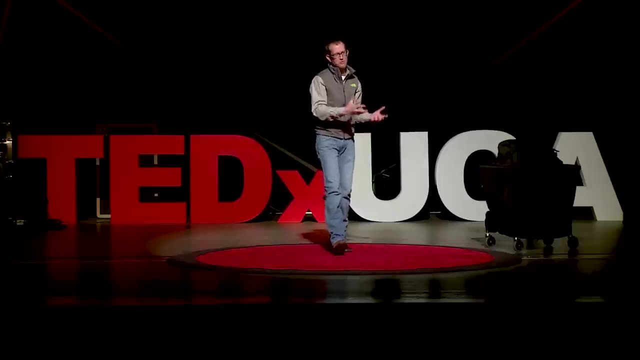 this turtle or this snake or this alligator or this salamander. I don't feel like everybody's looking at me. They're looking at the animal And I can relax And I can be a better teacher and not just a presenter. Appreciating those differences is so important- One of the best. 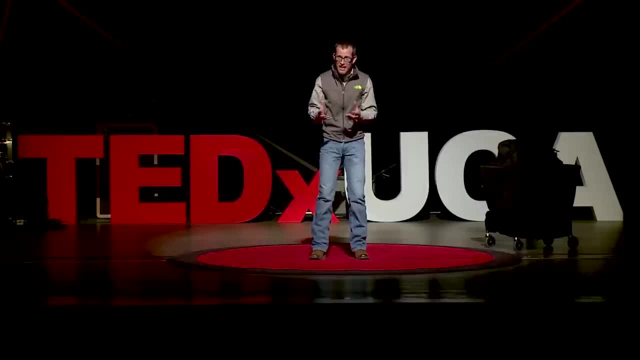 things that I've ever done at the University of Georgia through that class is have those students come together, take those animals and go about 10 miles down the road to extra special people. If you've never heard of extra special people, or ESP as we call it, let me tell you if you're in, that's. 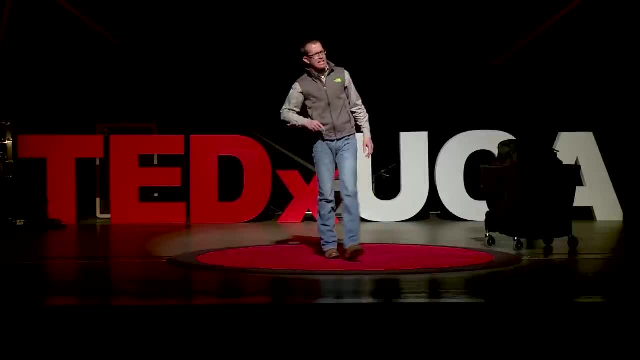 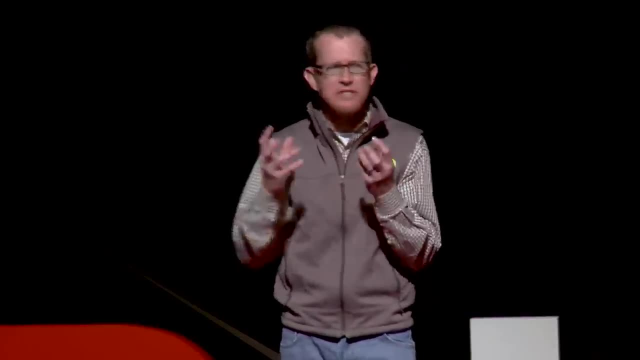 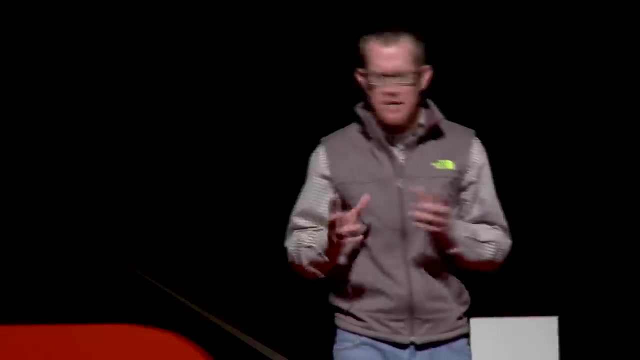 right. if you're in need of a hug, go on down to ESP. You will feel so welcomed and so appreciated. ESP is a place where literally hundreds of folks with disabilities, with learning issues, come together and they thrive. Special needs: They come together. I get my students with those animals. 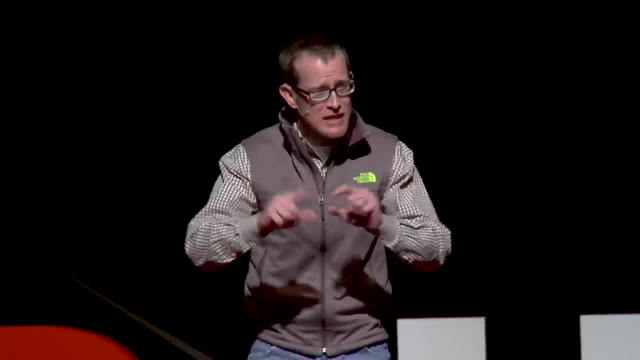 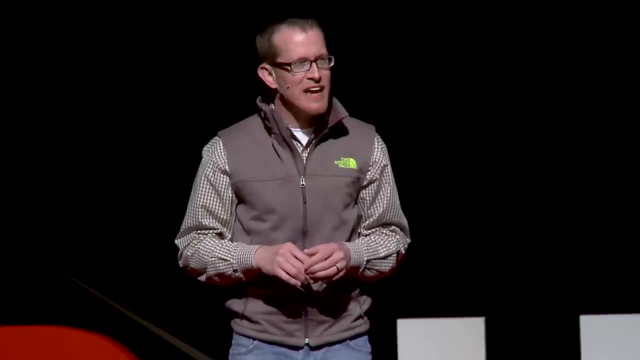 and some of those students are scared to death stand up in front of an audience and give a presentation And I get it. But they go to ESP And they see those faces- just like my student Dakota there, And they take that snake out or that turtle or that salamander. They. 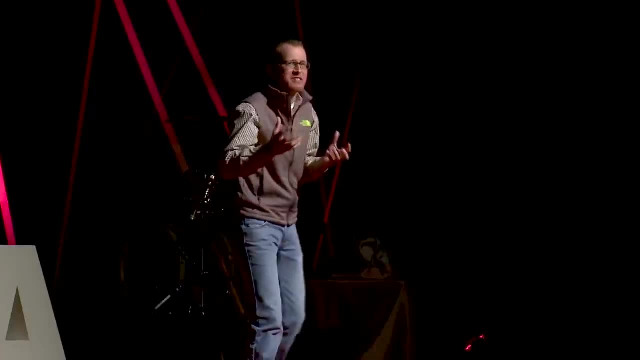 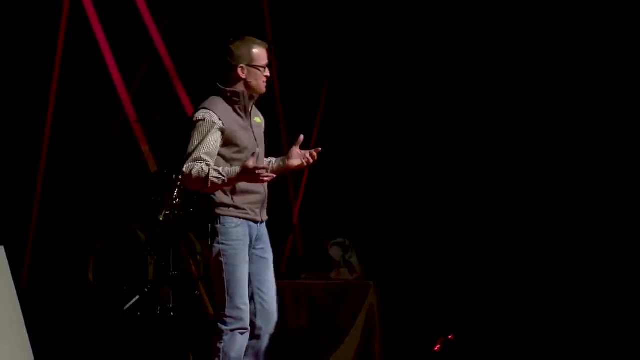 interact with those special needs kids and they see this difference that they can make. Those participants look at my students like they're celebrities. They come to ESP and they want to take pictures together. They know the animals. They know the animals by name And my students 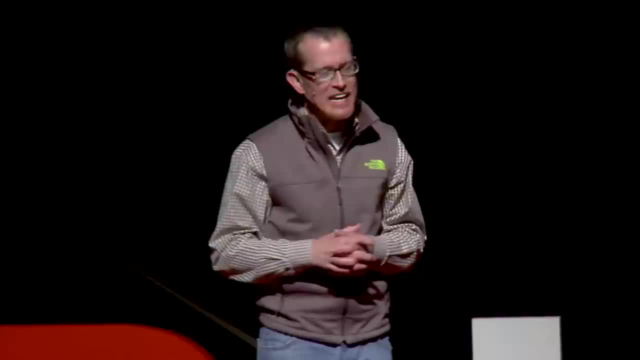 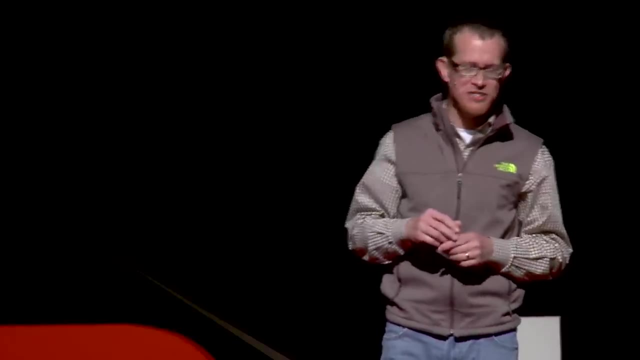 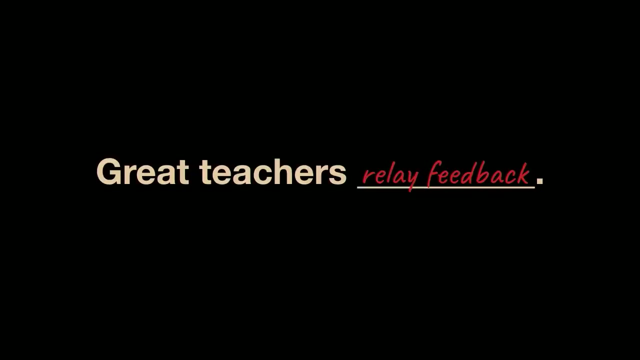 visit there and it builds their confidence Appreciating differences. Think about ESP. I tell you what an incredible organization. So the second thing great teachers do is they appreciate differences. The third thing that great teachers do, I think, is relay feedback. Now, when I'm in class, I can look out at my students and I can see if somebody might be. 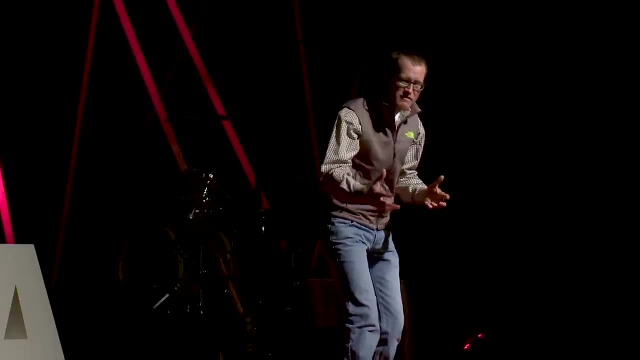 having a bad day or something's on their mind And I can ask them about it. Hey, how's everything going there? Give them a pat on the back, an attaboy, an attagirl, a fist bump, a high five. Everybody needs that. 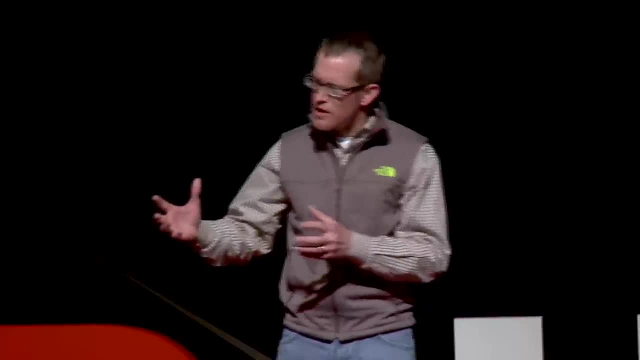 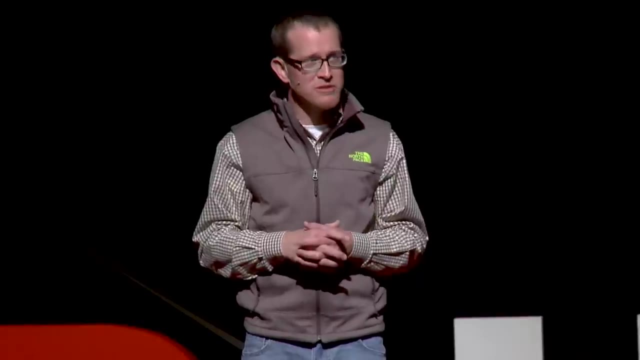 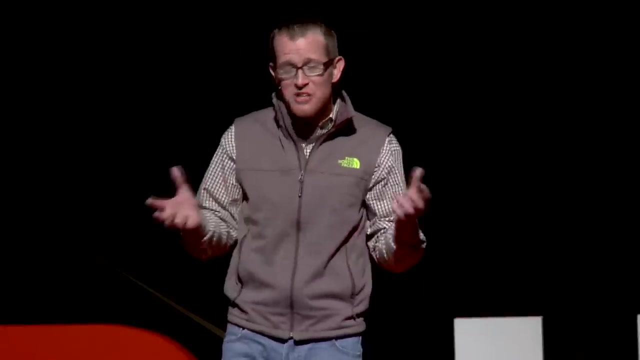 positive feedback. We're so sometimes caught up on negative things that we don't take time to say: hey, you did a good job on that. Well, students of mine know that I enjoy grading. Grading my assignments tells me how I'm doing as a teacher. 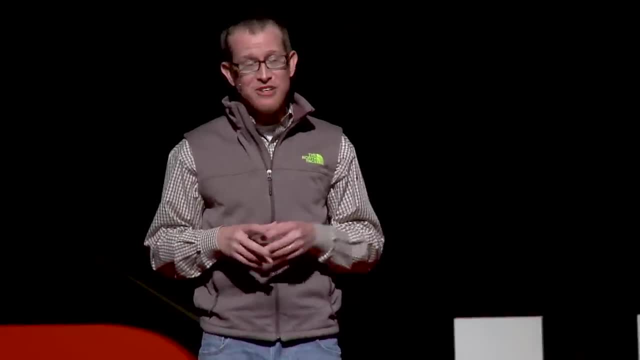 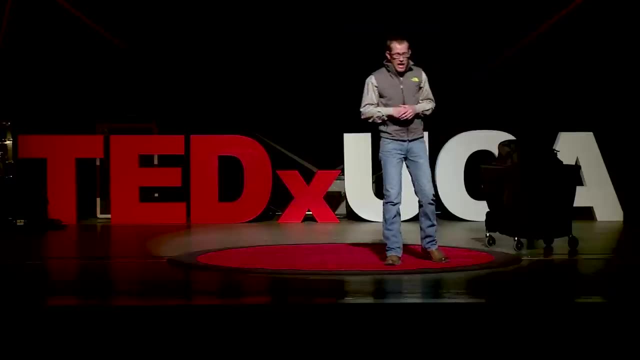 It's a really cool thing And my students know that if you get a 90% or above on one of my assignments, I put a stamp on it, And I have friends of mine that know that I do a lot of things And they tell me that I did something wrong, so I 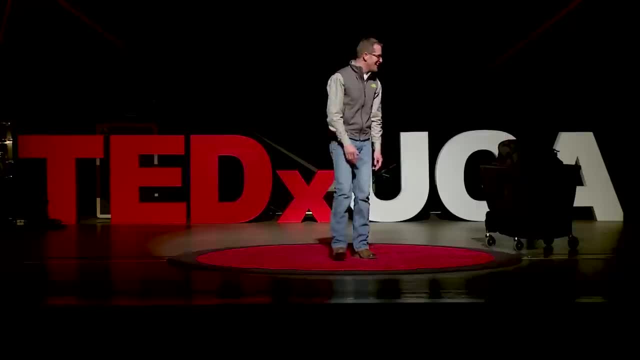 that I teach college and they say, Nick, I mean, they're not second graders, you're putting this asset. yeah, you get a ninety percent or above. I put a turtle stamp on there and I write: I write excellent job, I write it right on right. so and I do I. 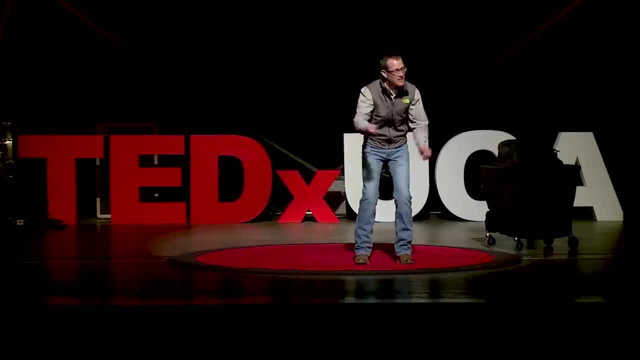 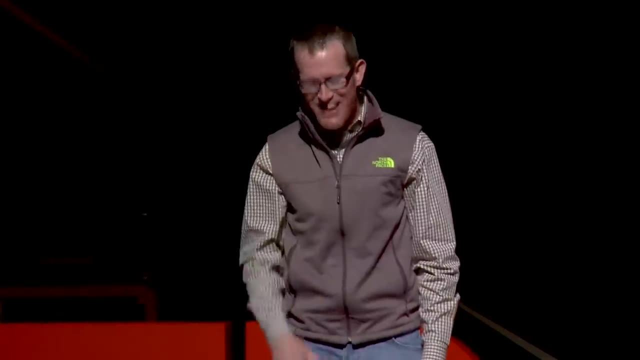 do that every time. people oh, come on and I look at their faces when I get it back. they're comparing: hey, I got a turtle on monitor. but the one time that I thought to myself: I don't know, Nick, you know I, maybe I could just grade them and hand. 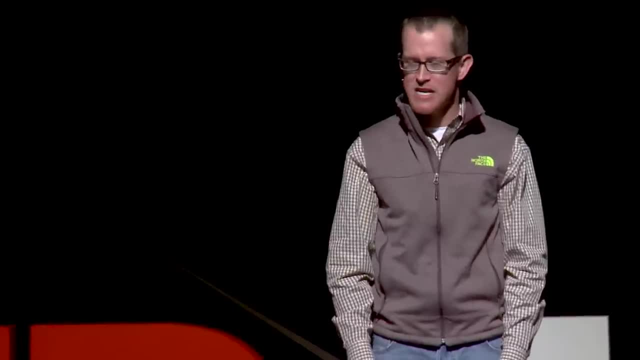 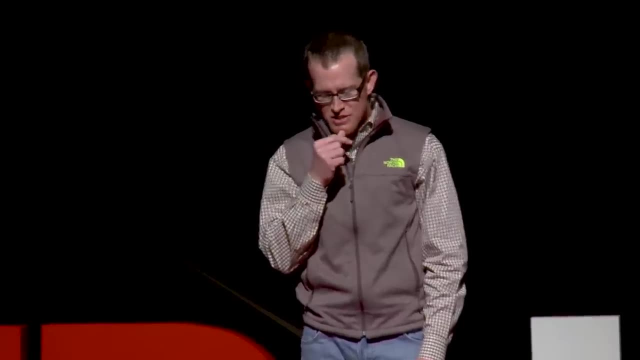 it back. it doesn't really matter. well, I tell you it does. I was teaching at a school to the south of here as a graduate student and it's a. it's a big university. it starts with an F, ends with Loretta. no, I know I'm not. 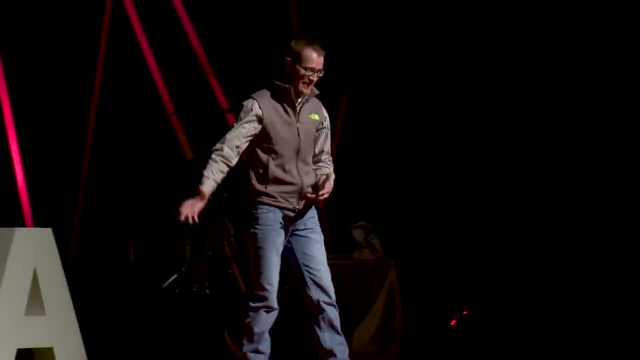 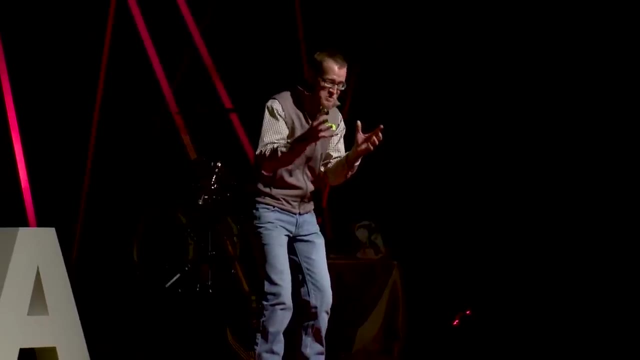 supposed to talk about it in Athens, Georgia, but I did go to school down there. there is credibility to this talk. all right, there really is. let's get out of here this guy. so I'm down there at that big University to the south of us and I'm teaching a big class as a PhD student. down there's a big class, a. 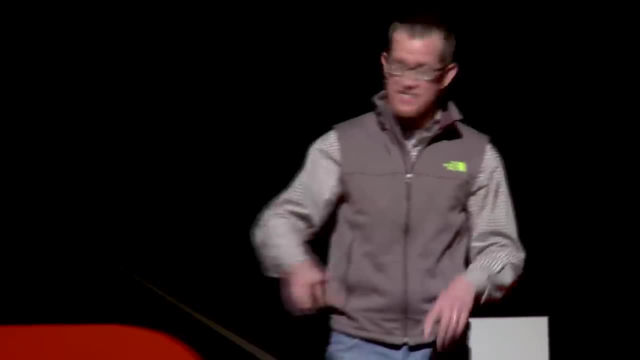 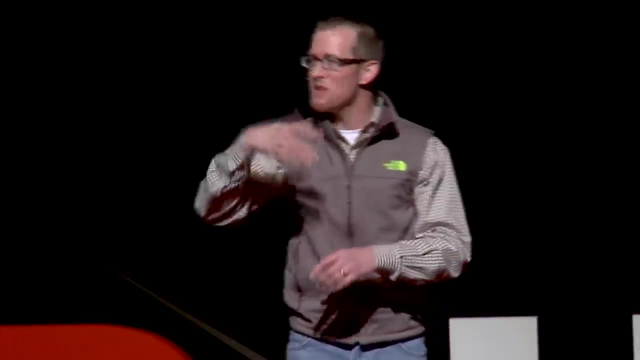 couple hundred students and a lot of football players would take this class and they would all sit down in the front down there and on day I was handed back assignments in class and I got done doing that, went back to my little cubicle as a grad student and I'm sitting there at my cubicle and there's 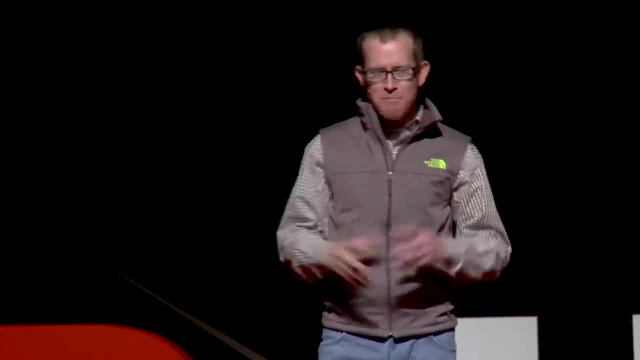 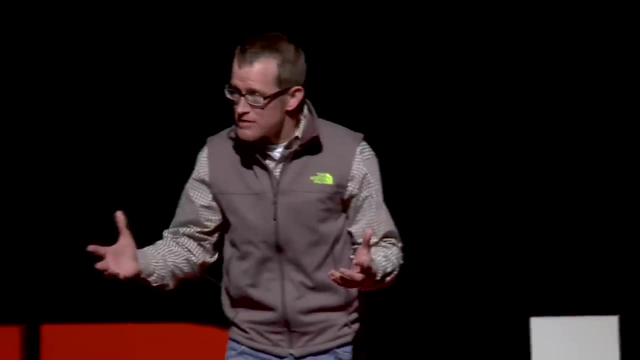 a knock on the door of the grad student office and I'm kind of back in a corner of this big office in my cubicle and I look around at the door and there's one of the football players, a linebacker, and he's literally- you look like a- 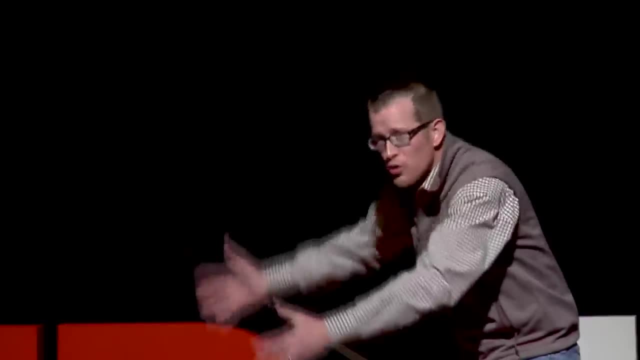 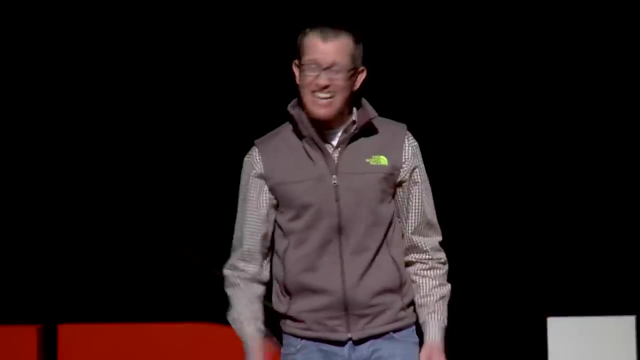 refrigerator. I mean the guy, he's taken up the whole door and and he's standing there and he's looking at me and he's got this assignment in his hand and it looked like a post-it note in his hand. I mean that's how big. and he's standing there. 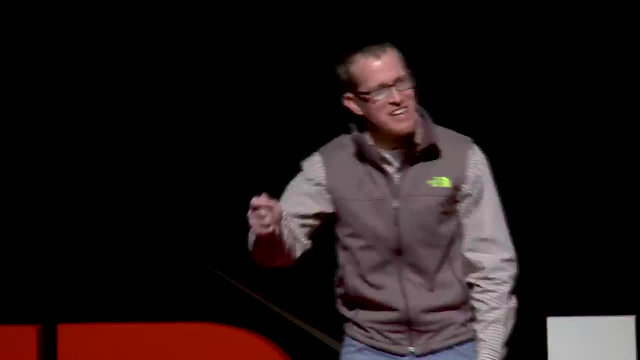 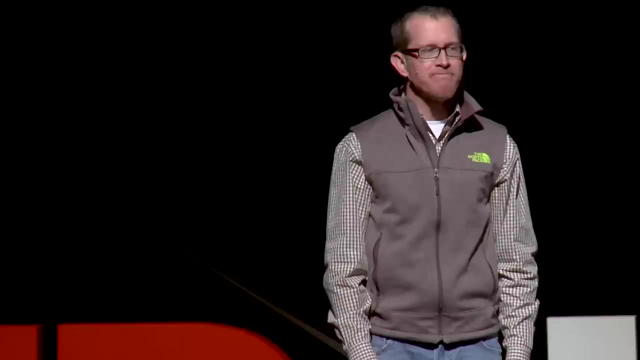 and he's standing there and he's looking at me and he's looking at me and he's got this: says: Ranger Nick, can I talk? And I love they call me Ranger Nick. Ranger Nick, can I talk to you? Come on in, Come on in. And he says: I got a 91 on this and I didn't get. 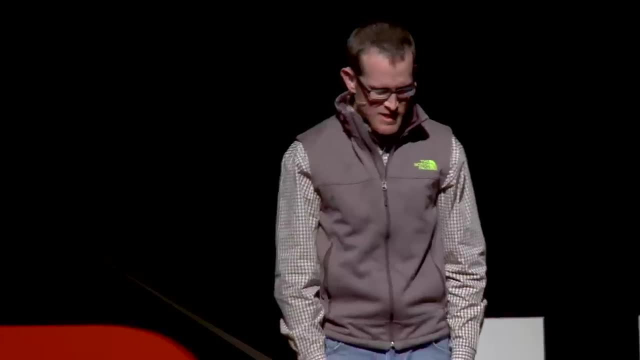 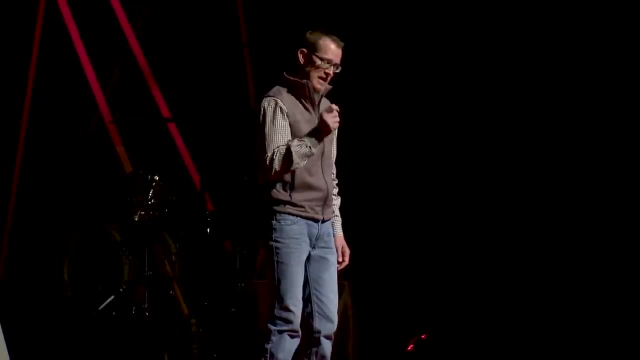 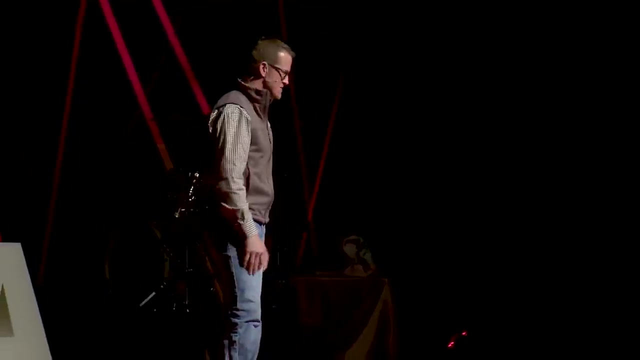 a stamp And I. he handed it to me and he, this guy, walked all the way across campus. you know, he came to the office and I'm looking at it- I'm sure enough I must've forgotten. So he hands it to me and I can still see this like it was yesterday. Hands it to me. I. 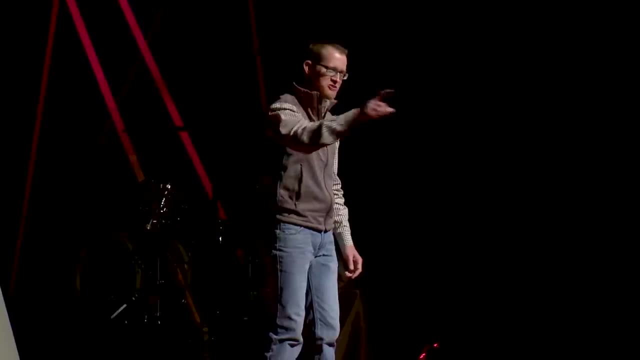 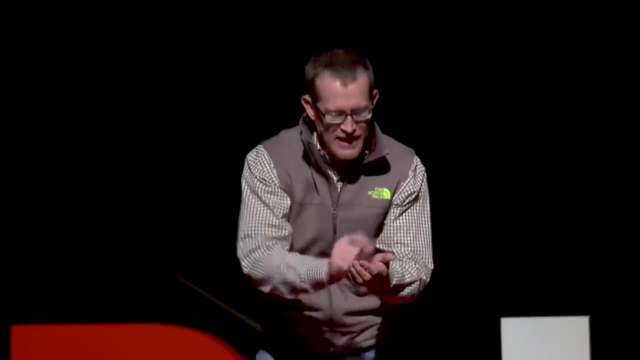 reach into my desk and I had an owl stamp in my desk. I still use today. My students that are here know this owl stamp. It's a legitimate owl, It is a good owl, And I took this little owl out and I inked it up and I stamped it on his page and I wrote owl standing. 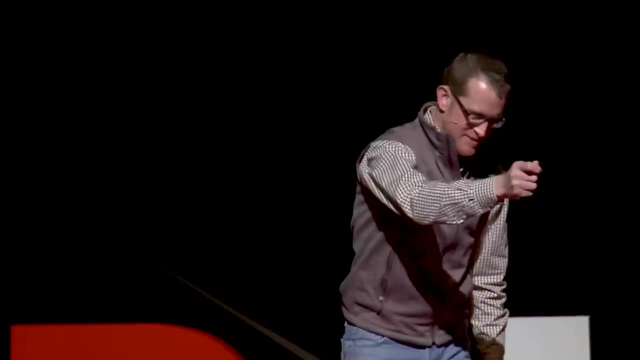 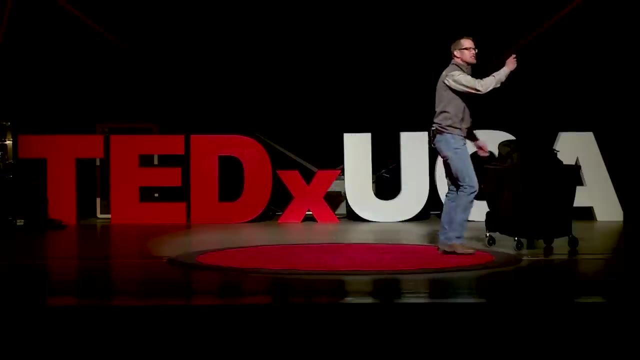 work And I handed it back to him And you know he walked out of there just as proud as smiling, like he was going to go show his mom, Ranger, Nick, I earned an owl stamp And I said to my friends who get on me about Nick: 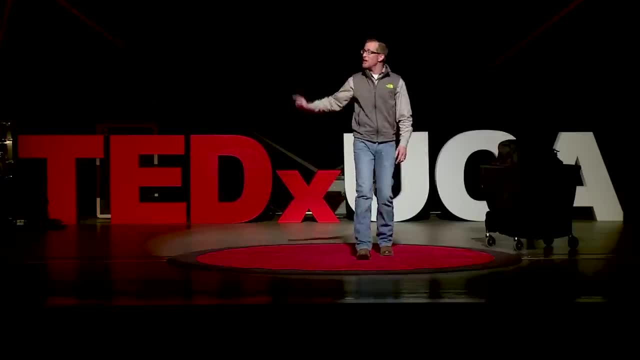 you know you give stamps. I said let me tell you if that big, tough football player could walk all the way across campus with that assignment to tell me he didn't get a stamp, wait to give me one. I'm going to do that until I retire from teaching. It matters. 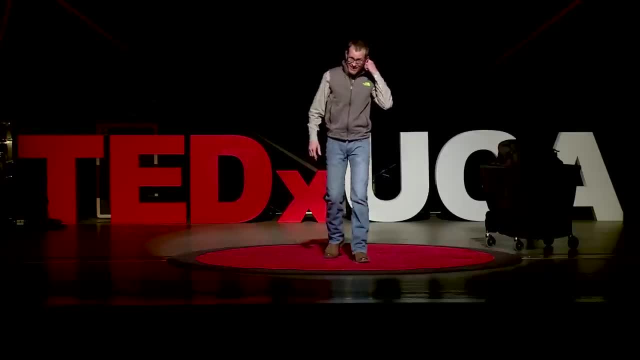 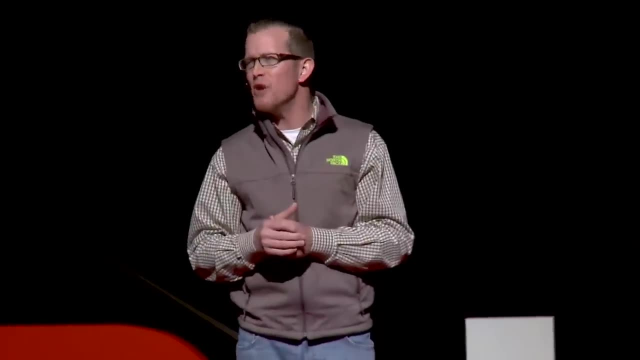 It matters. It matters, It really does. Relay and feedback: You've got to tell. you've got to tell people how you feel, man, you're doing a good job And that motivates them and they can't wait to do the next assignment. What other stamp will he use? I've got a leaf- unbelievable. 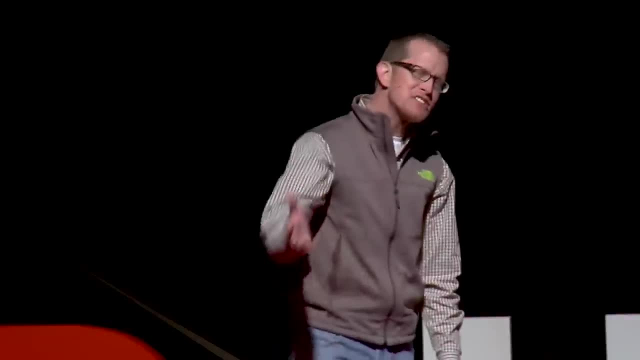 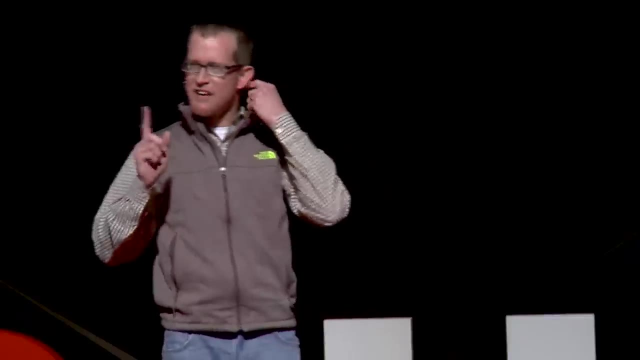 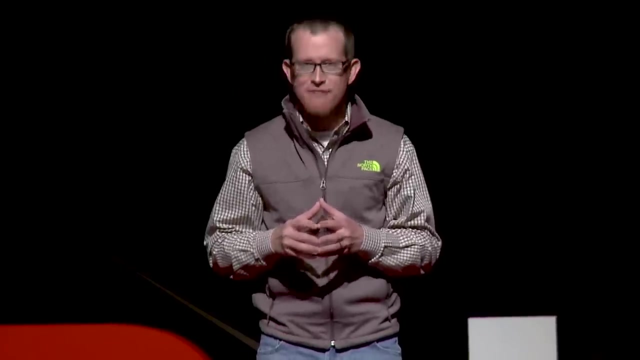 work If you're having some problems. I've got a paw positive improvement, These kind of things. Great teachers, relay feedback. I think that great teachers also- and this can be tough- they evaluate themselves And it's easy to take it personally. It's easy. 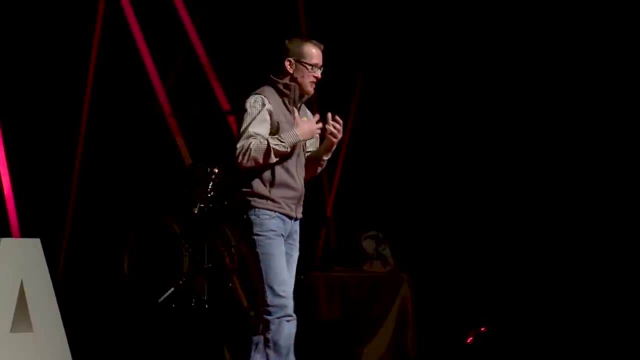 to look at that and say, oh, I don't know, I don't think they like me, you know. But you look at what students are telling you And you've got to be willing to change what you're doing if something's. 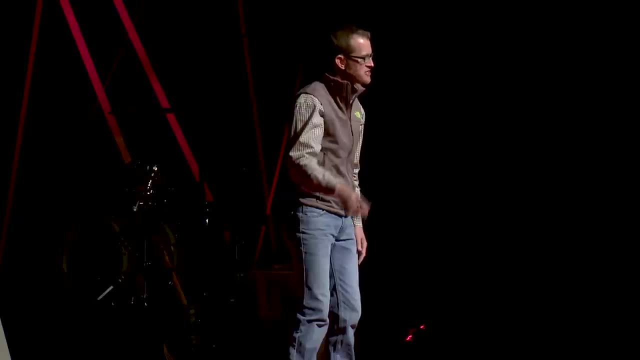 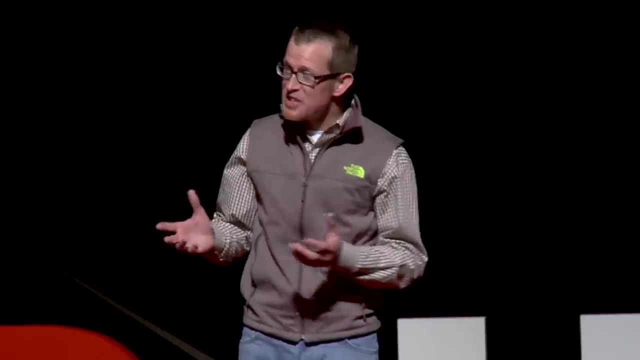 not working. You've got to look around the room at those facial expressions. You've got to look around the room at that body language. Do I need to change what I'm doing? It's important. Evaluating yourselves and your environment is really key, And I am sure that you're wondering. 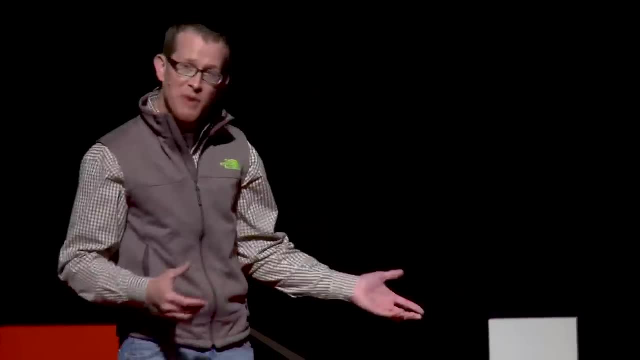 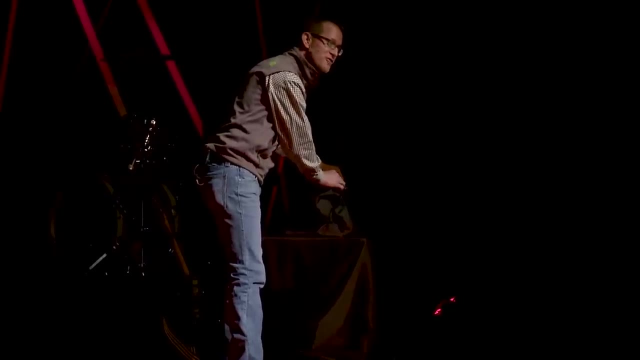 what is this black table doing here with this black bag on top- Which, by the way, I know that you all can't see it, But my wife gets me these bags and it says Ranger Nick on the front of it. It's kind of nice. She's here tonight, So inside. 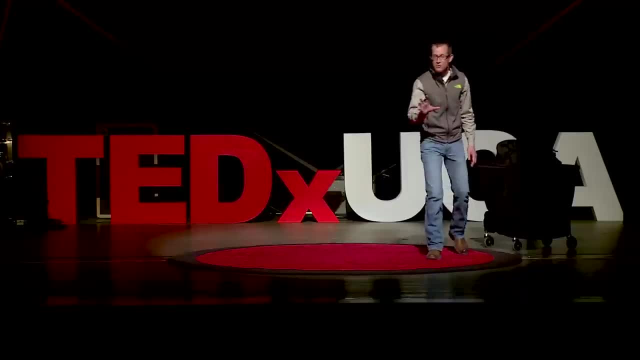 of this bag is something that does a really good job at evaluating its environment, And it uses multiple senses to do this. You know multiple pieces of data. So I'm going to reach into this bag and take this thing out And I promise, I promise it won't get away from. 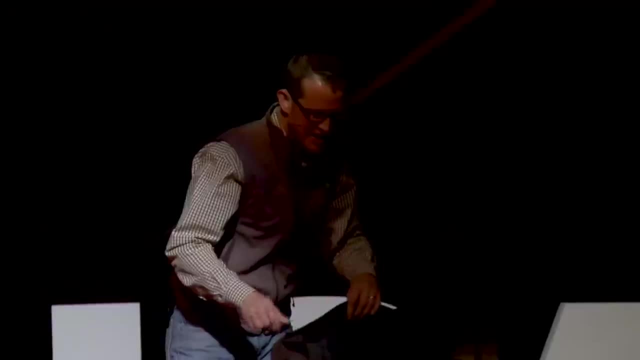 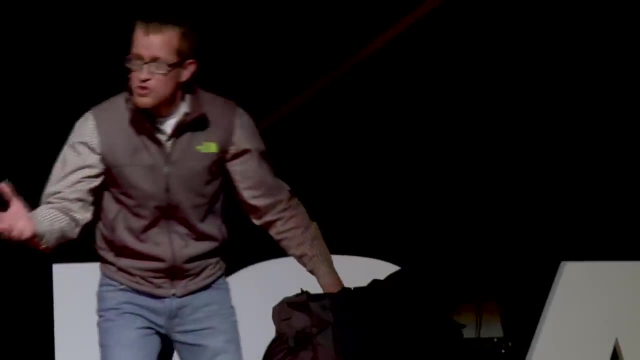 me. Okay, Promise, I'm going to hold onto this thing. Okay, It's inside of a bag, because it's a really good way to transport it. Plus, nobody knows what's in here. So when I'm at work over there at UGA and I've got a bag with me in a meeting and the bag starts moving. 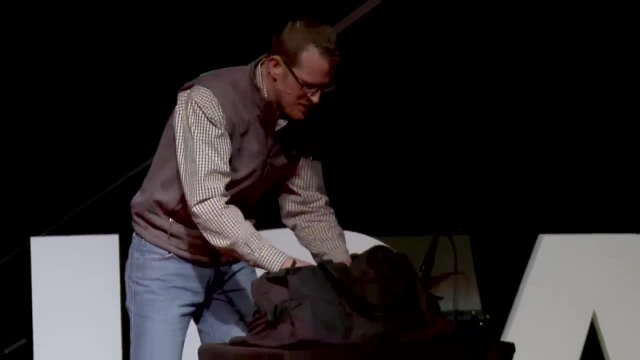 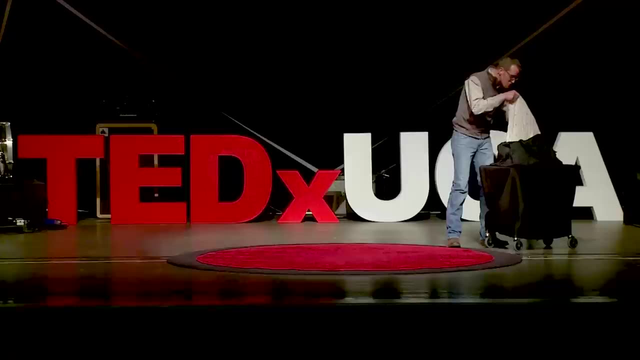 people, most people. what in the world has he got going on there? So I'm going to reach in here and I'm going to take a. I'm going to introduce her. She's called Snowy. Is her name Snowy? She is a sweetheart, She's a sweetie. Come here, girl. Let me show her. 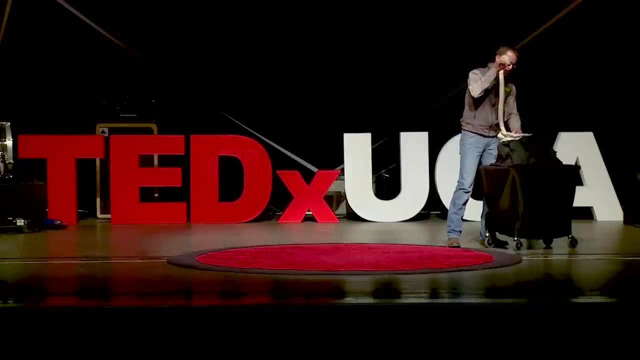 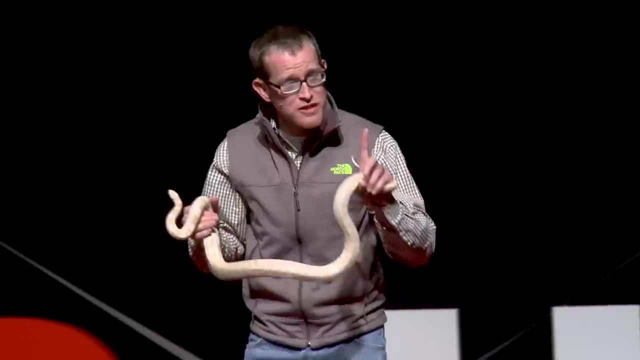 to you: Oh, she's all warmed up, ready to go. She's all. she's all warmed up and ready to go. Now I know what you're thinking And I appreciate that. nobody jumped up and ran away, You know. 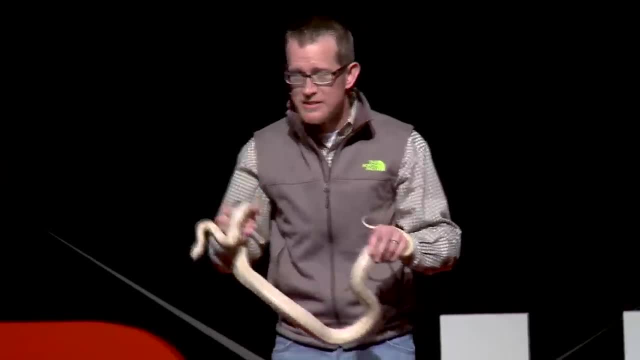 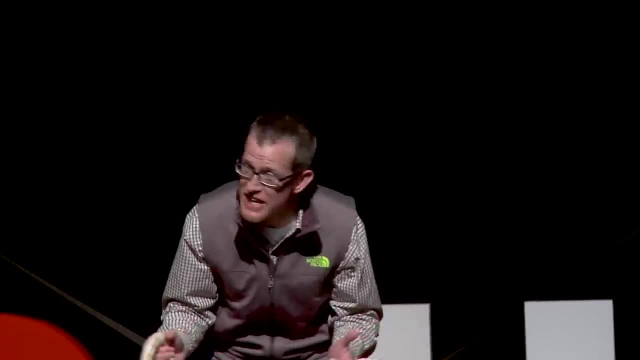 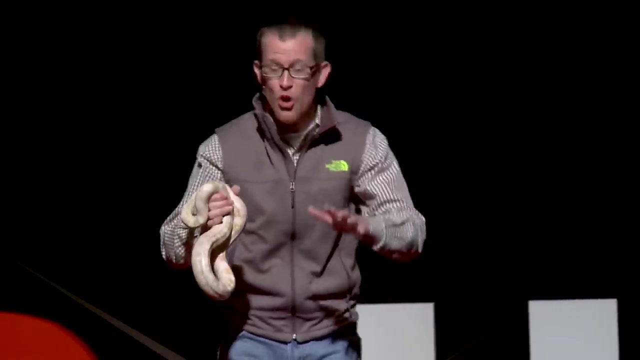 those football players were the first ones to run away. when I take a snake out, Tough guys, I know you're wondering. first thing, is it a poisonous snake? And first of all, there are no poisonous snakes. They're only venomous or non-venomous. This is a corn snake. 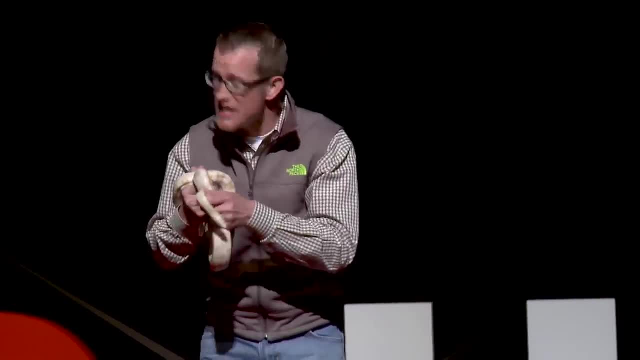 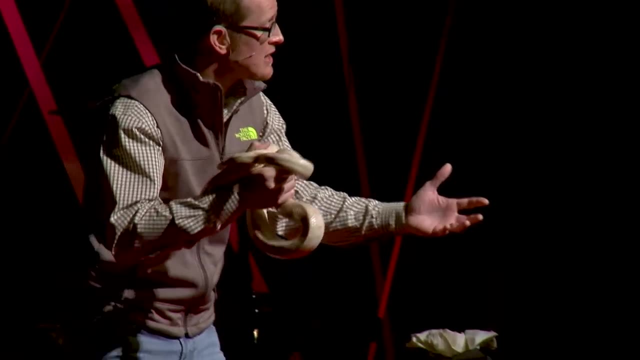 This is totally. they don't pay me enough to mess around with venomous snakes, So it's a non-venomous snake. It's non-venomous. Snowy is a corn snake. Snowy is a snow corn snake is what she's called. Beautiful little. 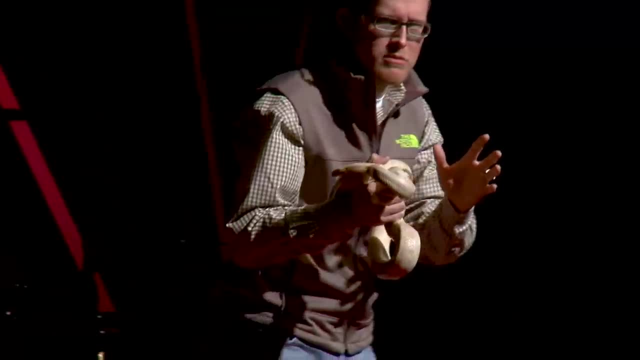 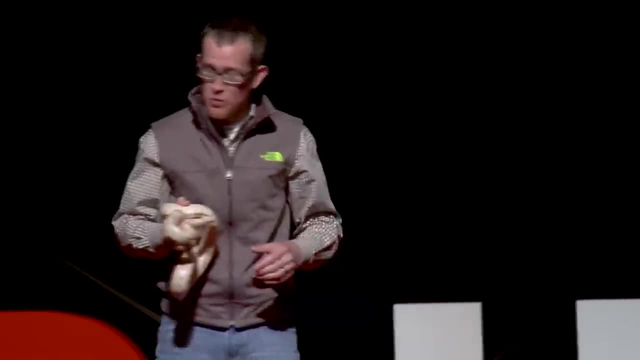 lady. Now this begs the question, though: How do you tell if a snake is venomous or not? You know, People ask me: what do you do? Well, if you look it up in some of these textbooks, here's what they tell you. First thing they say is look at the shape of their 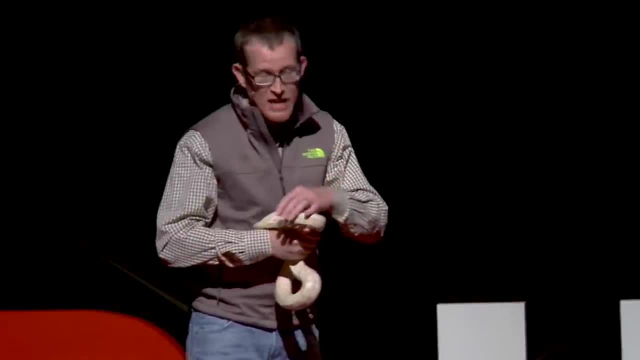 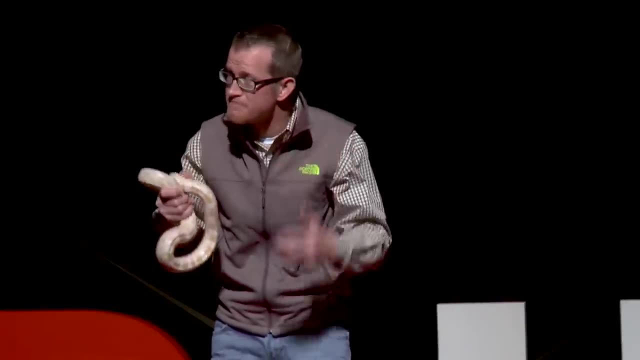 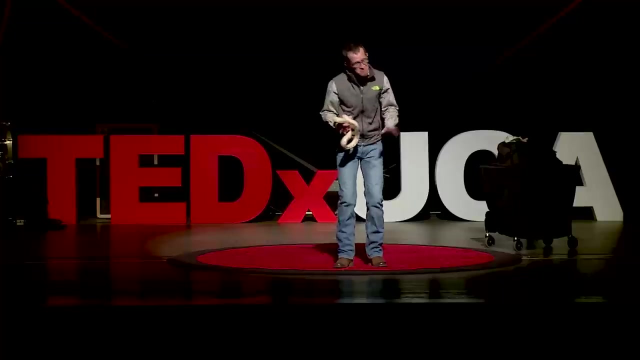 head. A non-venomous snake's head is an oval shape and a venomous snake's head is an oval shape. A snake's head is a triangular shape because of the venom glands back there. You gotta get kind of close to a snake to tell what shape head it has. Right, All right, Proceed. 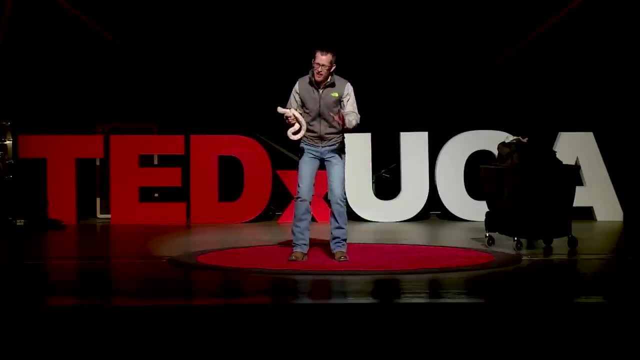 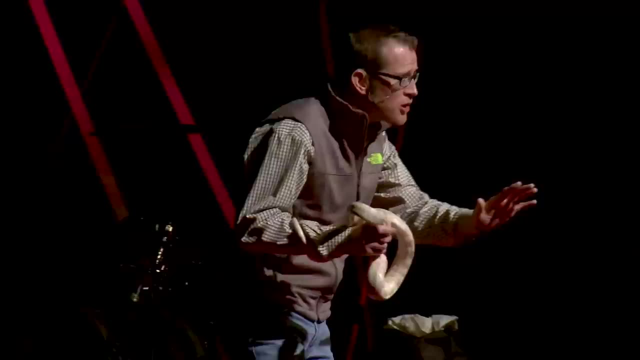 with caution, The next way I get to laughing about this. right, I get to laughing about this. yeah, The next way they say in the textbooks: the scientists, this is what they tell you. look at the shape of their eyes. 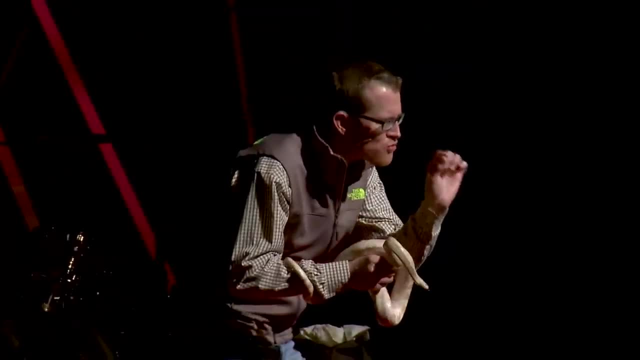 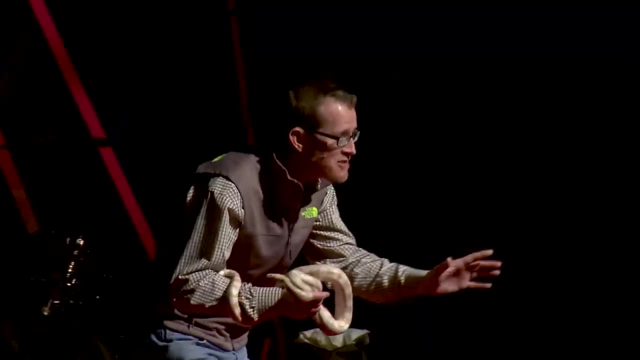 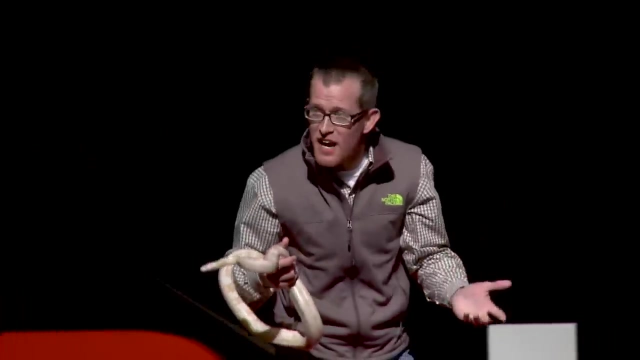 a non venomous snakes pupils are round and a venomous snakes pupils are vertical slits like a cat's eye. but can you imagine it, Bobby, get over here. Ranger Nick said: look at the shape of their eyes. is this thing venomous or not? by that time the things bitch on the nose, you know. so I always say when you 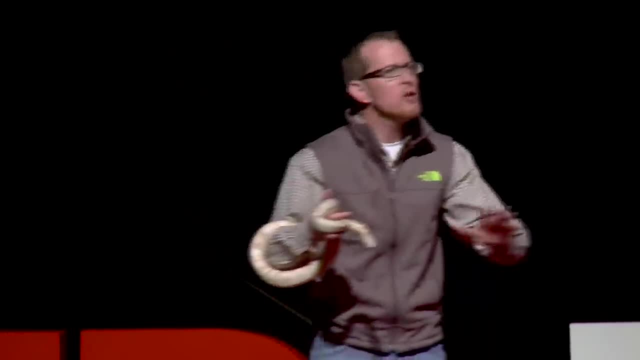 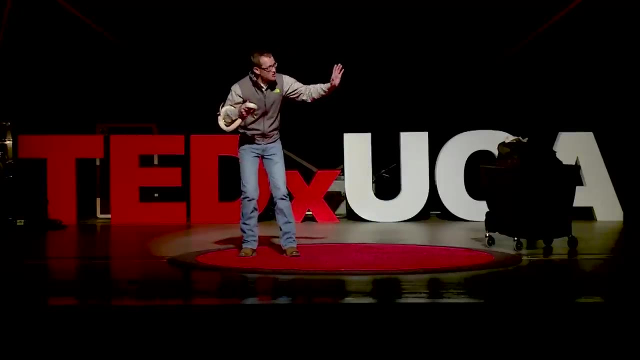 see something as beautiful as this out in the wild wave at it, say hey, thanks for what you're doing. don't get a shovel. don't jump up down and scream. appreciate what you're doing and walk away from it. they are doing incredible stuff out there to help us here in Georgia and all around the world deal. 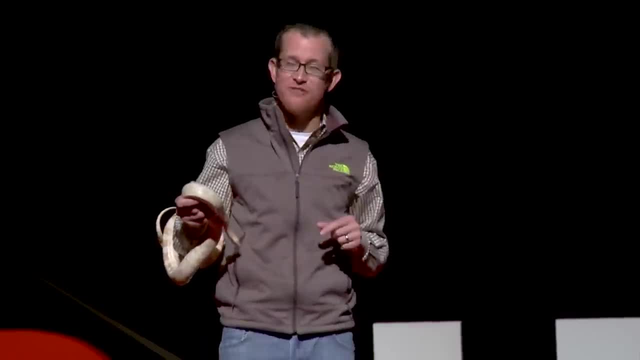 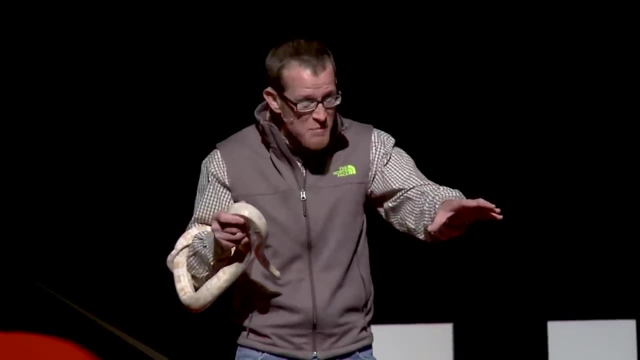 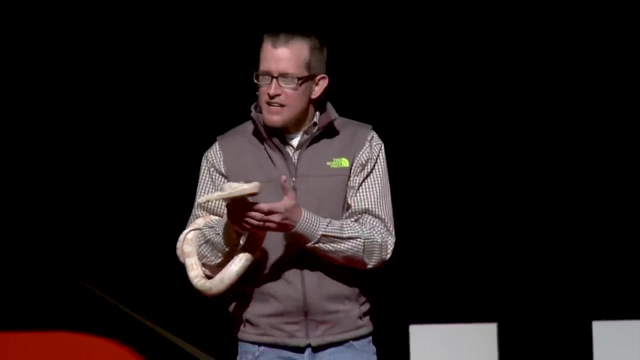 with rodents and things. snowy evaluates her environment just like all snakes do. that tongue is flickering in and out, tasting the air, wondering if anybody down in the front row has a mouse or a rat in their pocket. I hope you don't. she's about to eat again here soon. she's tasting the air, her belly senses. 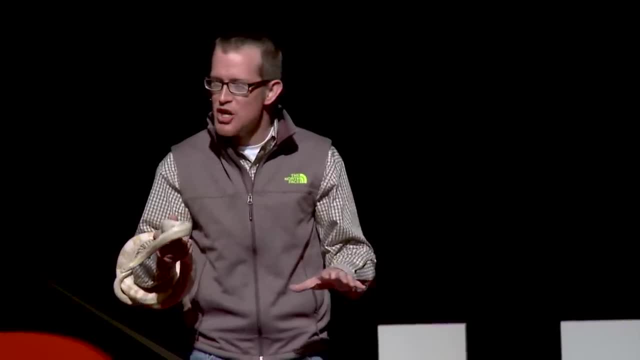 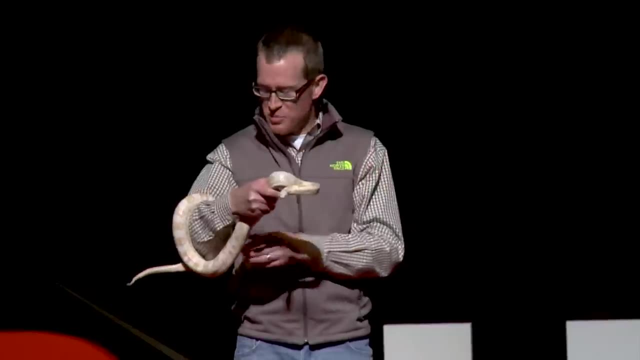 vibration. she's tasting the air. she's tasting the air. she's tasting the air vibrations. so when she's on the ground she can feel things. she's got this gland on the roof of her mouth that senses heat, because they hunt a lot at night. so all of these senses she puts together to determine her surroundings. where's food? 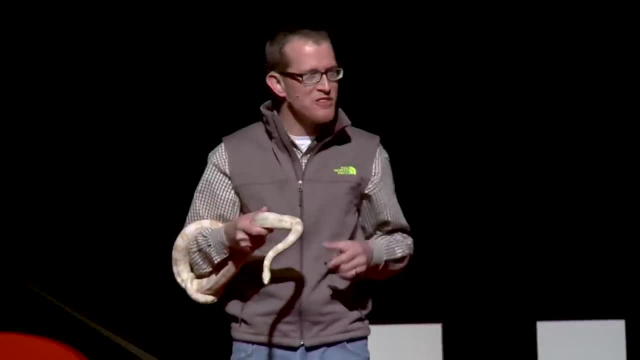 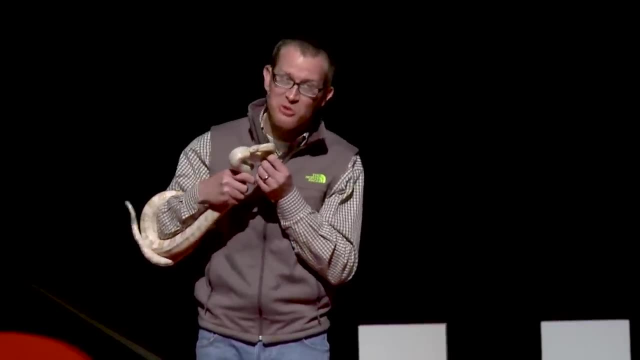 what's safe, what's not. same way, a great teacher evaluates themselves with multiple points of data to make a decision about how we're doing. snowy is a really, really cool lady and she lives at home with us in an aquarium. it's not loose, but she lives at home with us in an aquarium. it's not loose, but she lives at home. 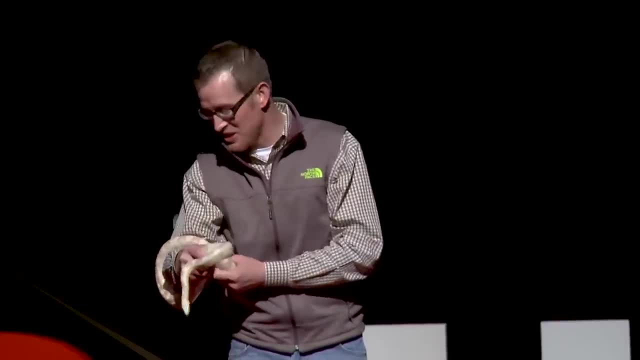 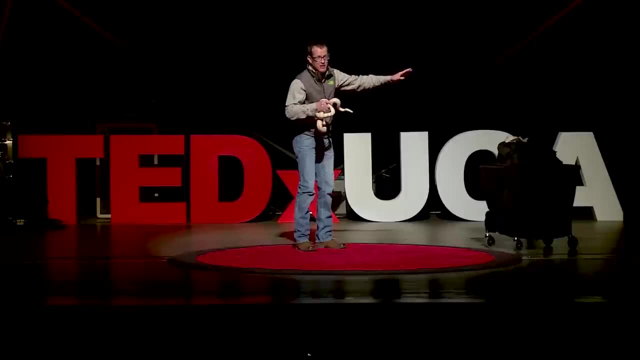 and those students at ESP know snowy very well. when I go to ESP they asked me about snowy. did you bring snowy today? she's a great one. I'm gonna ask miss Becca: come back out snake wrangler. she was a turtle herder, now she's snake. 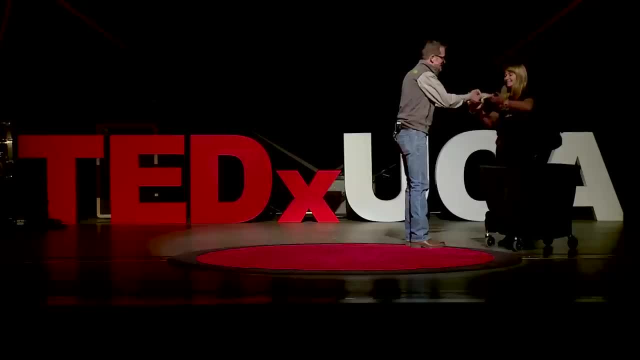 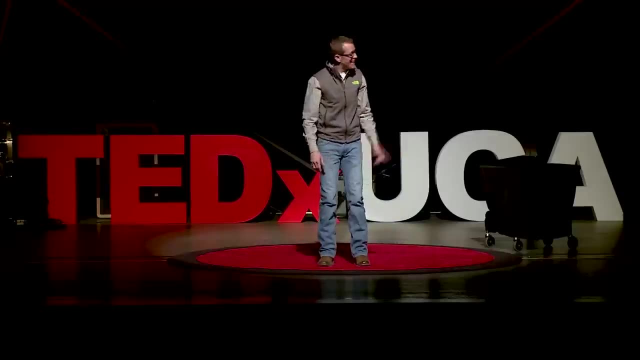 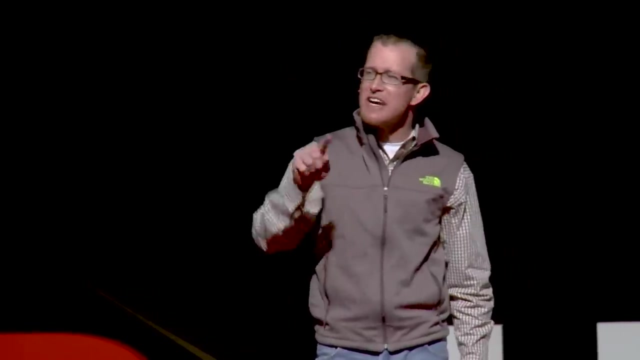 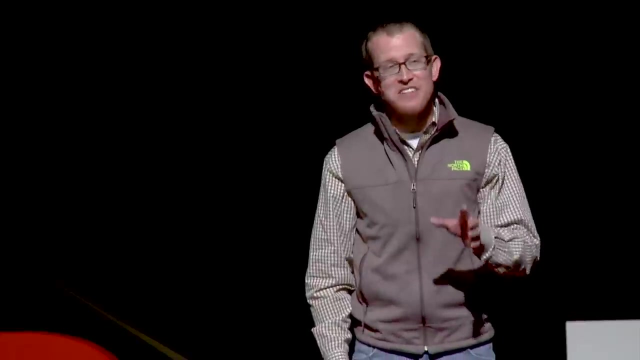 wrangler, can I give you a snowy. thank you, lady, so much. we'll give her a round of applause for taking care of that. that's great. think about what you put in that blank a couple years ago: great teachers, what I imagine that not too many of us in this room wrote down- that great teachers are the.